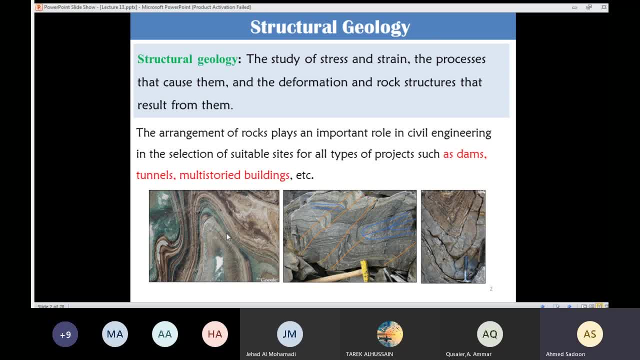 So, even if you don't get the concept of the stress and the strain from strings of material, I'm here to make it clear for you. So we said that today's topic is going to be about the crustal deformation, The deformation that is going to take place inside the crust. 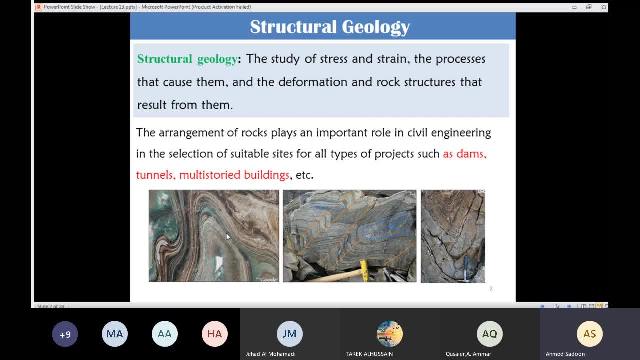 And in order to study this, it means that you are studying what's so-called structural geology. So structural geology means that you are studying the stress and the strain and any processes is going to cause them And, as a result, if you have, 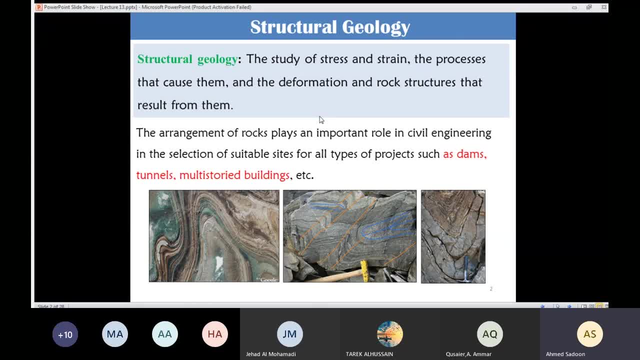 stress strain. that means you are going to have deformation And we need to understand what will happen to the rock after it's been subjected to stress and strain. So why studying the deformation? So the deformation of rocks is important for us as civil engineers. Well, in order to construct a dam, 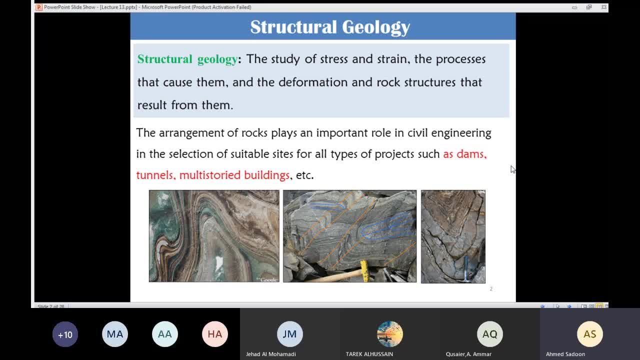 or tunnel or multi-story building. it's very important to learn, or it's very important to to know, the arrangement of rocks, Because if the arrangement of rock it is weak, at some point you may change the location of a dam or a location of a tunnel or a location of a multi-storied building. 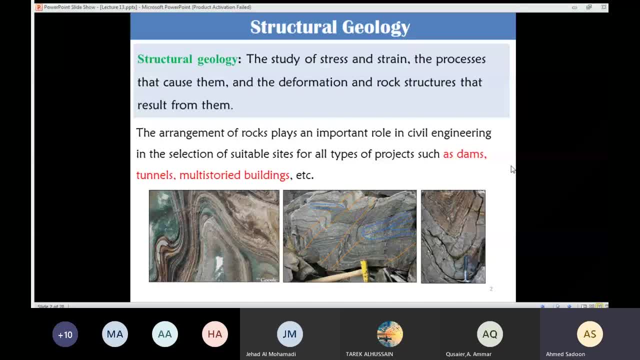 And in order to do this, you need to have good knowledge in soil mechanics. In soil mechanics, you are going to study everything about the soil, And rock is going to be considered a type of soil, So the arrangement of soil is very important. 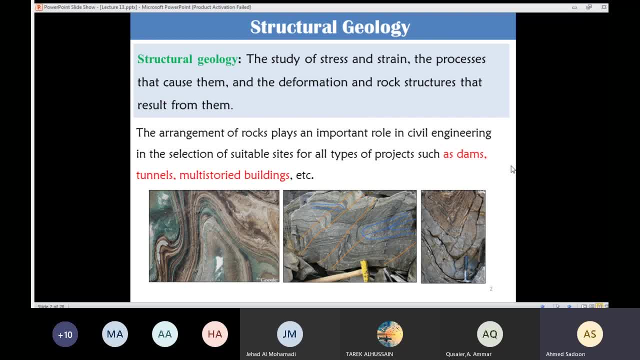 And the structure of the soil, whether it's being subjected to stress and strain, is very important. In order to have a decision about the location of a dam or tunnel or any civil engineering projects, it's important to know the structure of the rock and the arrangement of the rock. 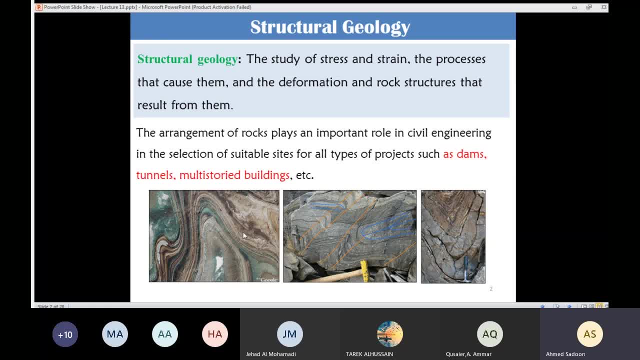 Like you can see in the pictures here, you see a rock here and here and here And it's clear that These rocks were subjected to stresses from the pictures, Because we are seeing a lot of deformation inside the rocks. Today we are going to understand this type of deformation. 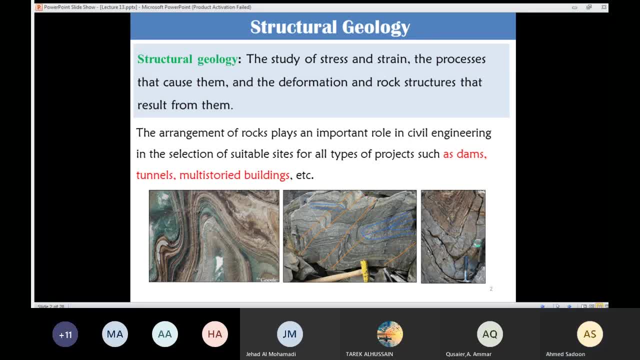 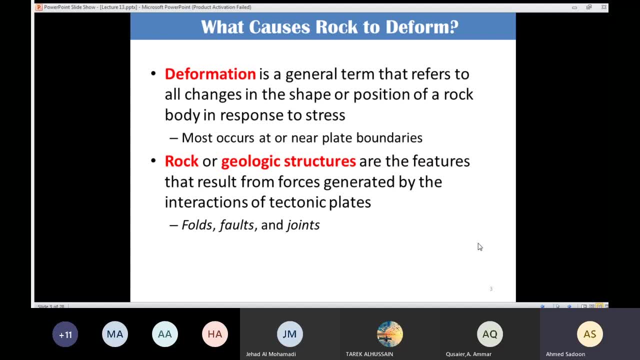 But first, when we say deformation, it's a general term, It's not specific, just a general term. It refers to all changes in the shape and the position of a rock. So if you have changes in the shape or if you have changes in the position of the rock, 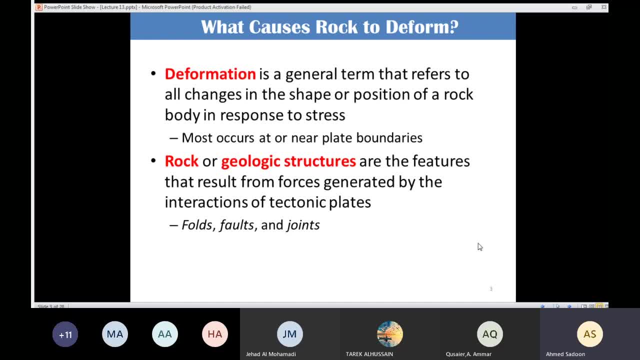 because of the stress we are going to say, we have deformation in general. And in order to have deformation, like I said, we need to have stress. And, as you might have guessed, you will know that in order to have stresses, the stresses, 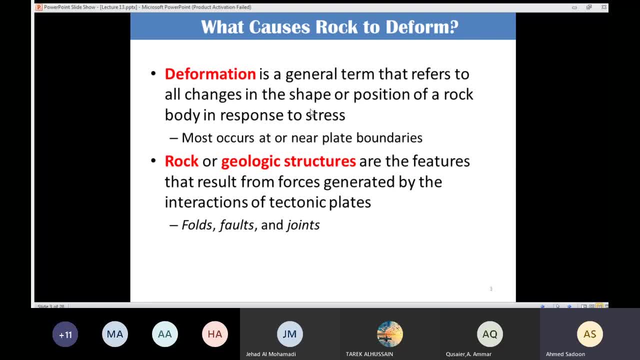 must occur at or near the plate boundaries. why do you think the stress is going to take place at or near plate boundaries? anyone can guess the answer: because of the type of the movements. they either- uh, go against each other, yes, yes, which means that you are going to have stress. so most of the deformation is going to take place at. 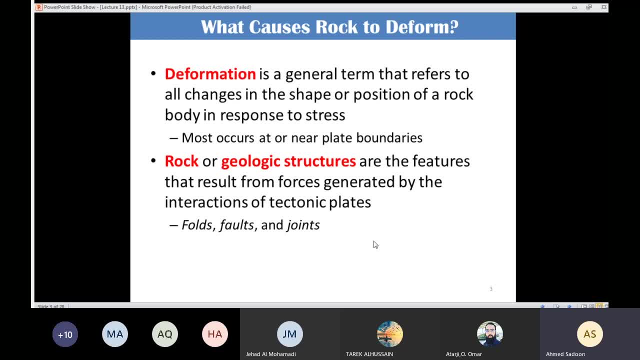 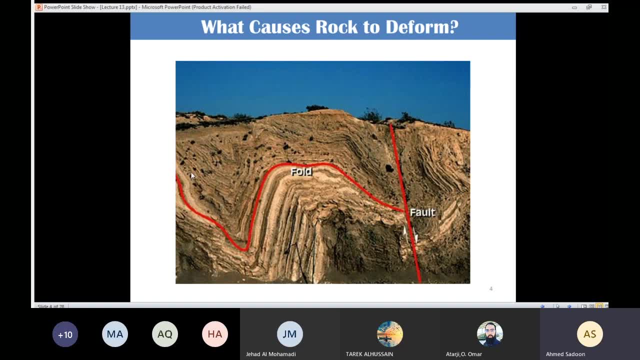 or near the plate boundaries, and if you have something like that here, as you can see, we have a group of rocks here which is clearly it has been subjected to stresses, and we call this. for example, if you have something like waves, condensed like waves like that, we are called this fault. and if you have fracture like this one and if you have relative, 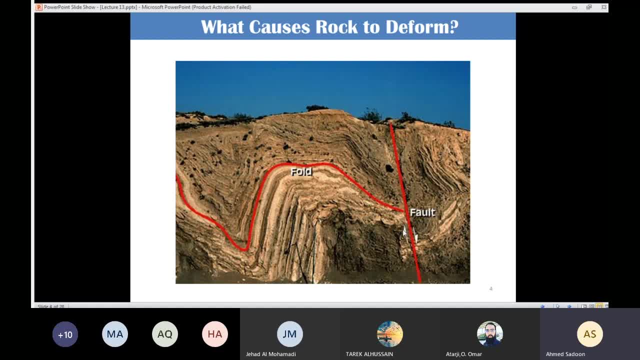 movement. if you have fracture with relative movement, which means that the position of that point it should be here. but when i have fracture like this one plus relative movement, we we are going to call this fault. so if you have a fault or fault, we are going to say: 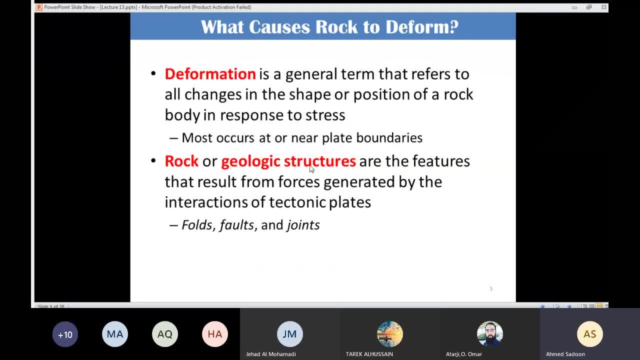 that we have rock structure or geologic structure, geologic structure, so geologic structure, are the features that result from the forces. so here we have features resulted from the forces and we know that the forces it has been generated by the interactions of tectonic plates. so faults, faults. 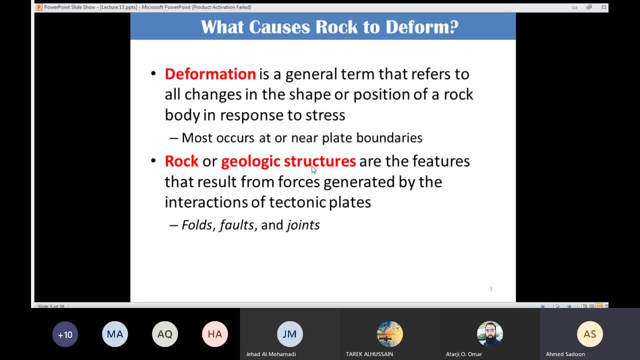 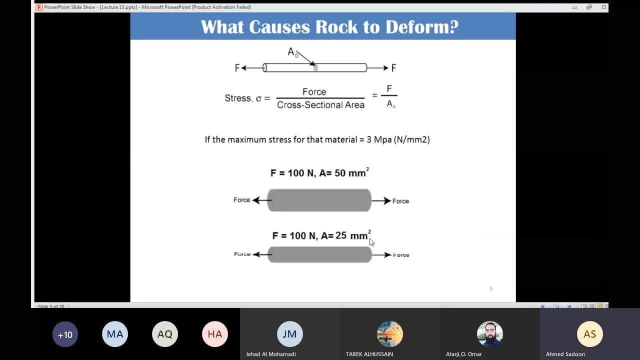 joints are geologic structure or rock structure. okay, and in order to understand the stresses, i'm going to give you simple example. first, we need to ask ourselves: why do we need the term stress? so, mathematically, stress equal force over the cross sectional area, if you are looking. 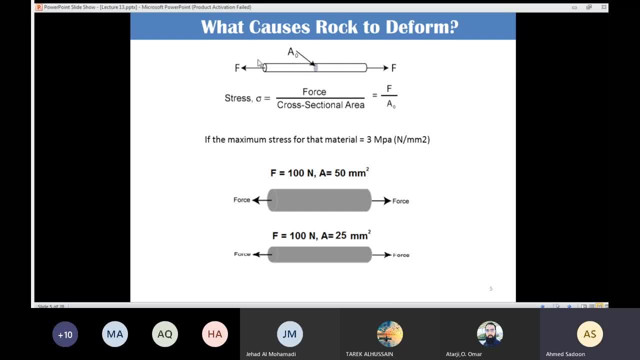 at this rod here which is subjected to force- force f and so force f- and it has cross-sectional area. so the cross-sectional area here it's mean the area which is perpendicular to the force. so the force is here and that area is perpendicular to the force. 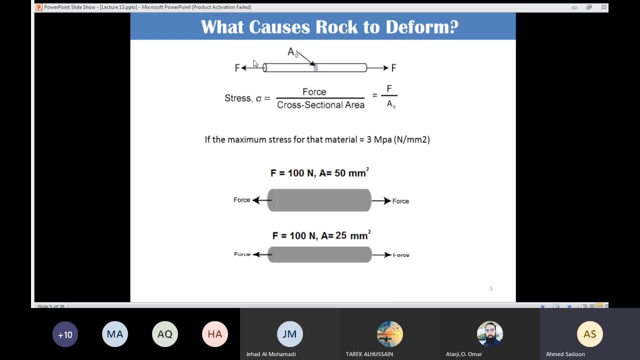 so this one is going to be considered as cross-sectional area. so in order to calculate this stress, you need to know the force and you need to know the structural, the cross sectional area. so stress equal f over a and the stress in the most of the textbook are referred to by the 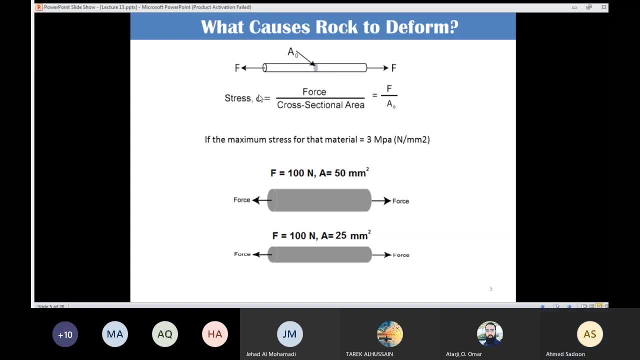 letter or the greek letter sigma. so sigma equal f over a naught. f represent the force and a naught represent the cross-sectional area. again why stress is important to understand this. assume that the maximum stress for this material here equals three megapascal. you know that megapascal it's mean newton per meter cube. 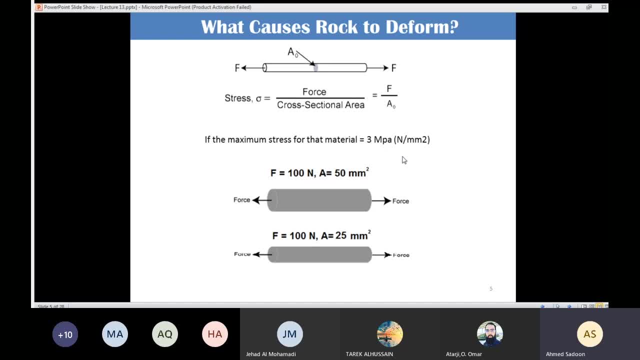 if we are going to say that the maximum stress equals three megapascal, if the material is subjected to stress more than three megapascal, what will happen to the material? it will fail before. yes, it will fail, it will fracture, failure will take place. and if the material is subjected to stress lower than the maximum stress, lower than three, 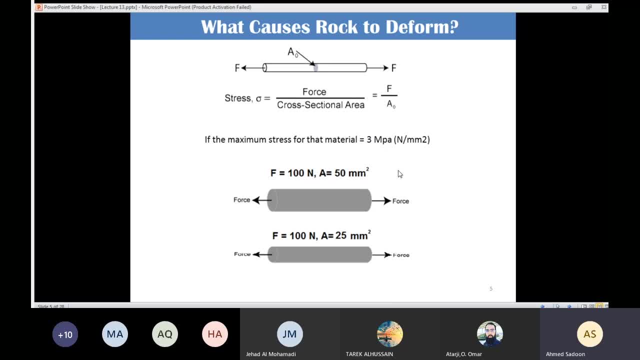 megapascal. in that case, what will happen to the material? will it fail or it will stay holding? and the material is subjected to stress lower than three megapascal. in that case, what will happen to the material? will it fail or it will stay holding? the obvious answer is: the material is not. 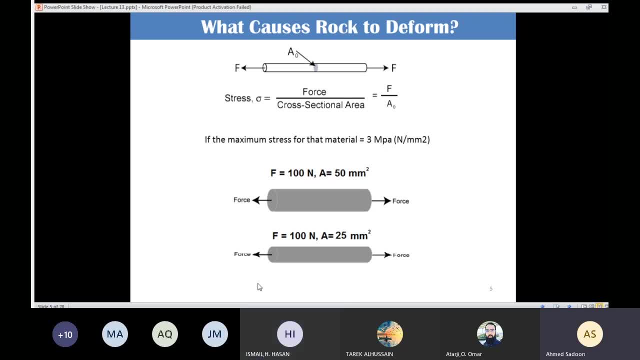 is not going to fail. yes, because the stress is lower than the maximum stress. so here, assume i have road number one and road number two and they are made from the same material. so here, assume i have road number one and road number two and they are made from the same material. 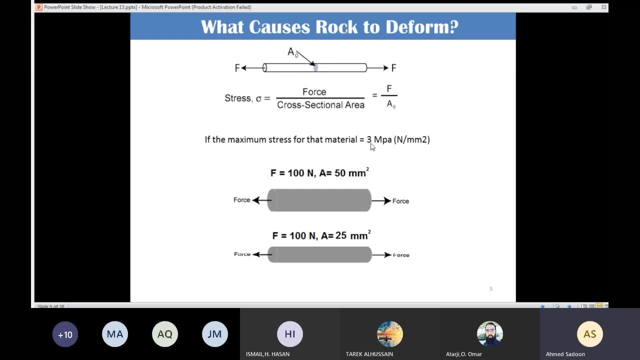 so here assume i have road number one and road number two and they are made from the same material with maximum stresses equals three megapascal. okay, so i have road one and road two. in road one the force equal 100 newton. in road 2 we have the same force, which is 100 newton. 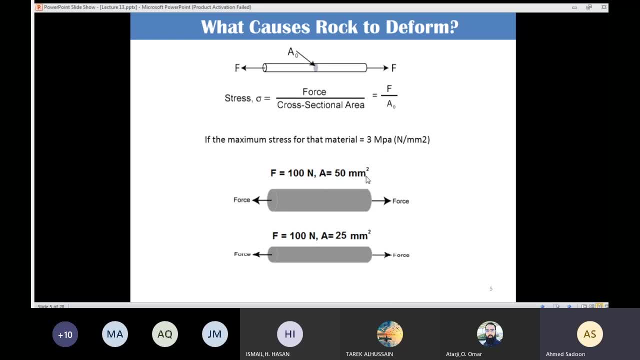 in road one, the area equals 50 millimeter square, while in road 2, the area equals 25 millimeter square. So we have the same force, but we have different area, different cross-sectional area, So which one is going to fail? 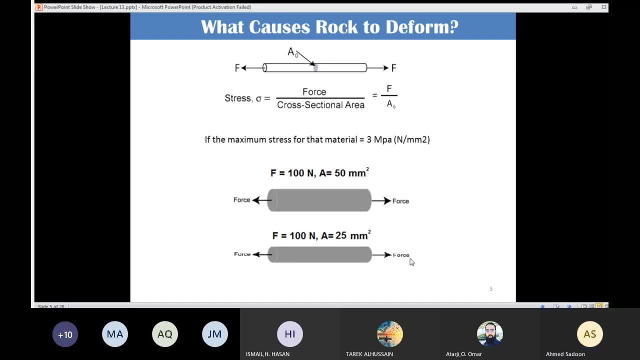 Road 1 or Road 2?? Road 2, doctor. Road 2 is going to fail. Why is Road 2 going to fail? We have the same force, No, but the area is different, and we have a rule called B equals F over A. 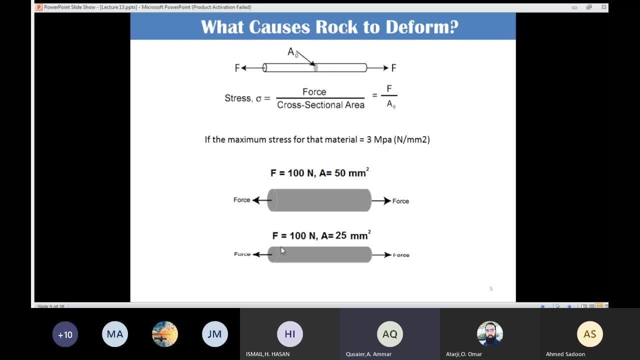 when we have a big. I can't say it, Doctor, if you have, Yes, you are saying. You are saying that you are going to calculate the stress here And the stress here in road number 2 is higher than road number 1.. Yes, that's what I mean. 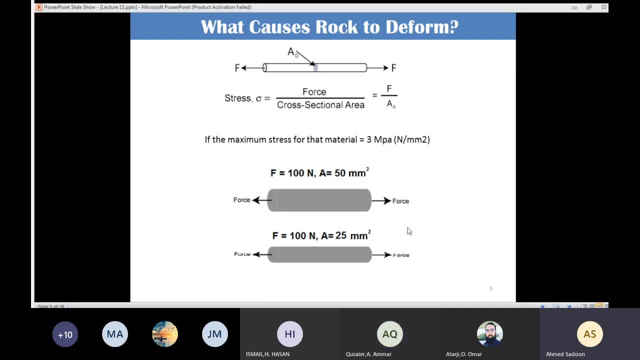 But why road number 2 is going to fail? You already proved that road number 2, it has higher level of stress than road number 1.. But why road number 2 is going to fail? Because it's more than 3 MPa. It's going to be 4.. 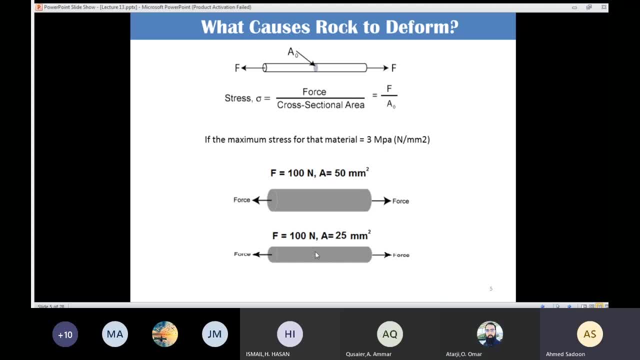 Yes, excellent The stress here. if you calculate the stress here, you are going to say that sigma equals F over A, Then it will equal 100 N over 25 mm2.. So the answer: it will be 4 MPa. 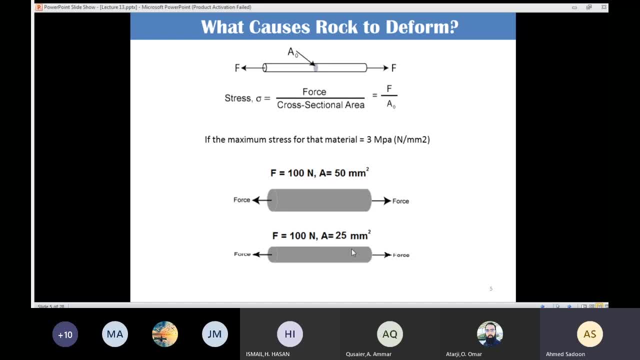 And 4 MPa is higher than 3 MPa, Which means that road number 2 is subjected to stresses more than it can take And, as a result, failure will take place in road 2.. If I'm going to define the material by the forces here: 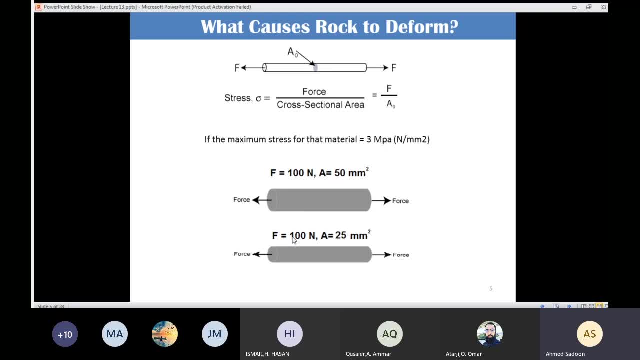 for example, if I wanted to buy some material- let's say you are going to buy steel- then will you ask about the force or the area? Or I'm going to buy the material depends on its strength. These stresses And why. 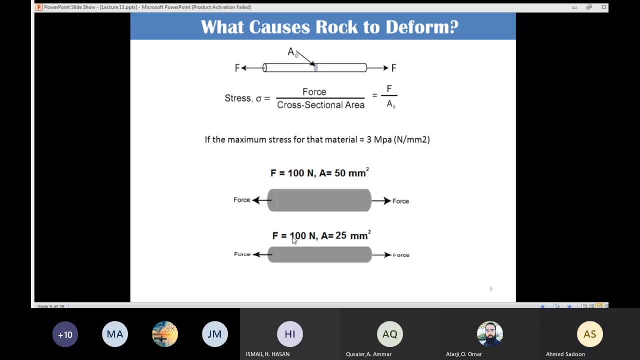 Did you understand my question? I will buy it according to the value of the stress that it can hold. why, why not the force? because the force may vary. it's not the problem. if I know how much stress it can take, I can apply multiple values of the force on it. yes, 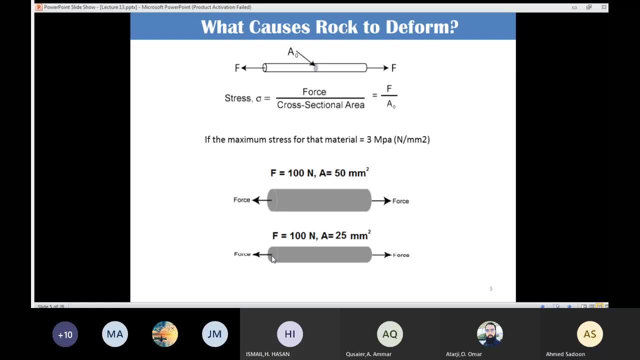 that is. that is the reason why- because you cannot buy the material by the force, because maybe the material can take a lot of force but the area is going to be very large or the area could be very small. so we need to relation between the force and the area in order to buy the material, and that ratio is known as. 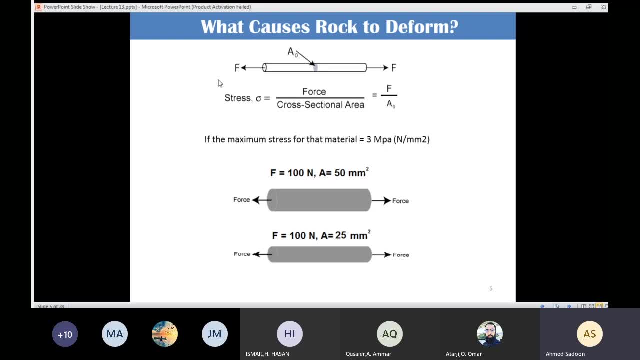 stress. so that is why stress is very important. I cannot buy a material by how much force it can take or how much area does it have, but I'm going to buy a material by stress, whatever the cross-sectional area. it has been a practice for all civil engineers to buy materials by the 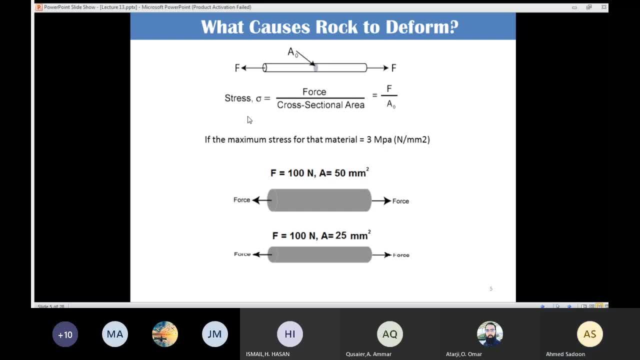 stresses and the strain. so now we understand the concept of the stress, why we have a stress, how to calculate the stress, why stress is very important and the rocks is going to subject it to stress and, as a result, we are going to have deformation. so stress is a force that deform rocks. 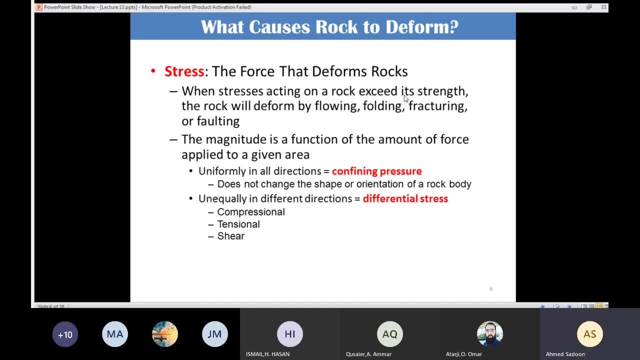 and also when stress is acting on a rock, exceed its strength, the rock will deform by flowing, floating, fracturing or faulty, which means that some kind of failure is going to take place because the stress is more than the its ultimate capacity and we know that the magnitude of the stress is a function of the 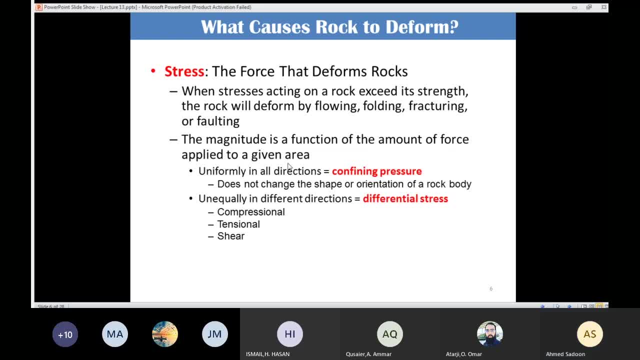 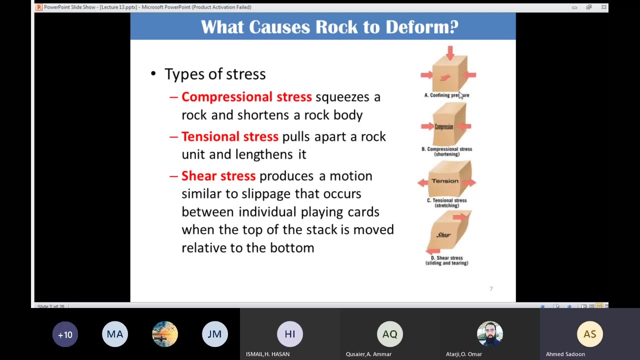 amount of the force applied to a given area. we already discussed this in the concept in the previous slide, by the previous example, and we need to know that this stress it could be uniform from all directions. for example, if you have cube like this one, the cube, of course the cube- you can say any kind of 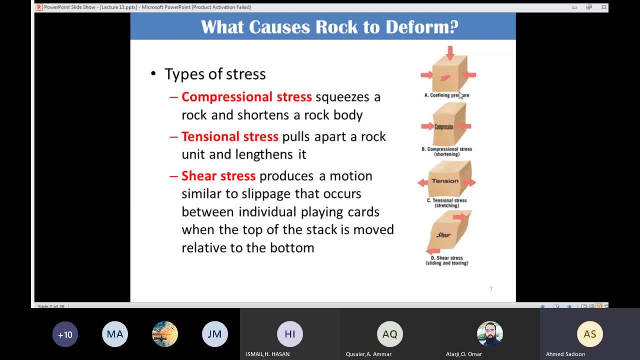 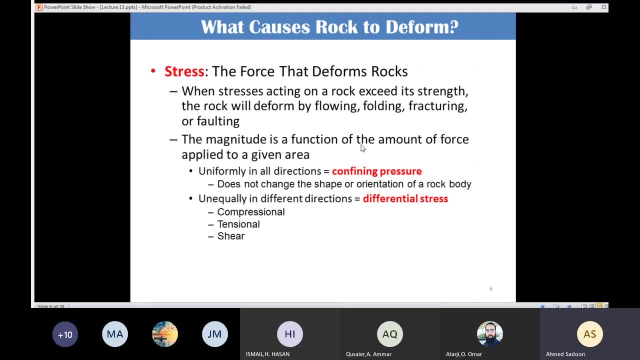 material. but here we are going to talk about the rock. so if you have a cube here made from rock and it's subjected to stresses from all directions, the stress is here equal to stress here and here and here. in that case we are going to say that we are having confined pressure. so confined pressure, it means 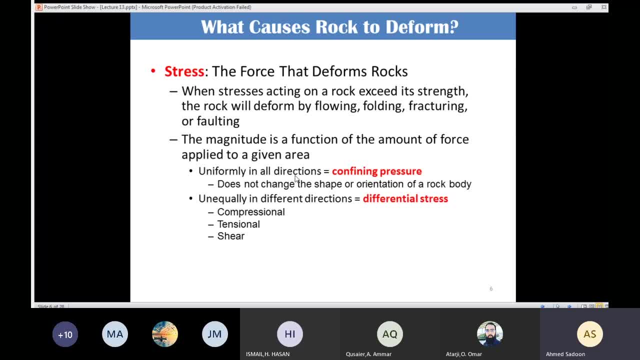 the stress is uniformly distributed in all directions and, as a result, we are not going to have a change in the shape or the orientation of the rock body. the differential stresses, on the other hand, it means that you are going to have a stress which is distributed and equally in different directions. so this means 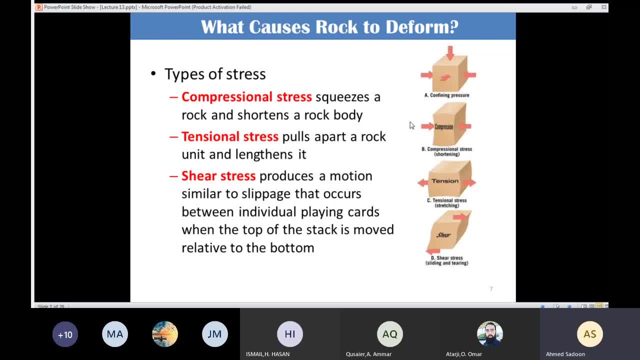 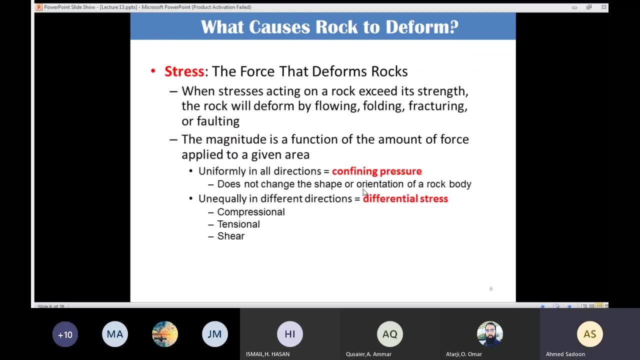 that if I have cube like this one, the stress in that direction is higher than that direction and or lower than that direction. the main point is the stresses in one direction is different than the stresses in the other direction, and in that case we are going to say that we are we are having differential stress. so 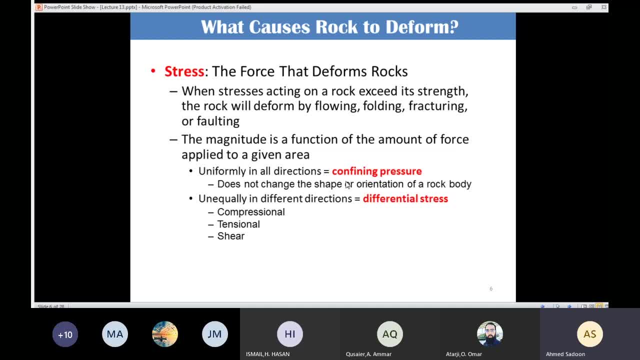 the stress. it could be confining or it could be differential. if it's equally distributed in all direction, you are going to say that we are going to have confining pressure if it's distributed and equally in different direction, then we are going to say that we are having differential stress and the differential 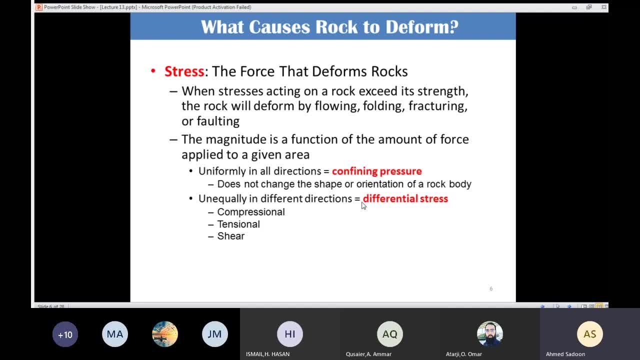 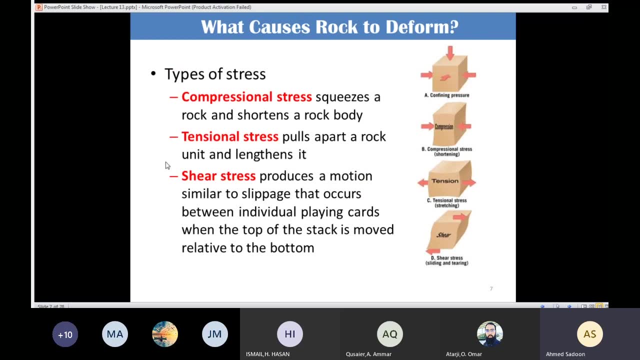 stresses. it could be divided, divided into three main categories. we have the Com師lon E differential stress. we have tensional differential stress, we have shear differential stress. so, the differential stress, it could be compressional stress, could be tensional stress, could be shear stress. so, if you have compressional stress, that means i'm going to squeeze the rock. 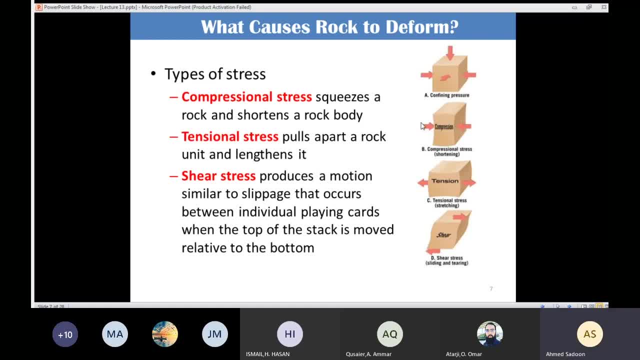 for example, if this one is a rock, by having forces in this direction and in that direction, i'm going to squeeze the rock, to compress the rock and of course, as a result, the direction of the force here is going to be shorter than the other direction. so compressional stresses, squeezes a rock and 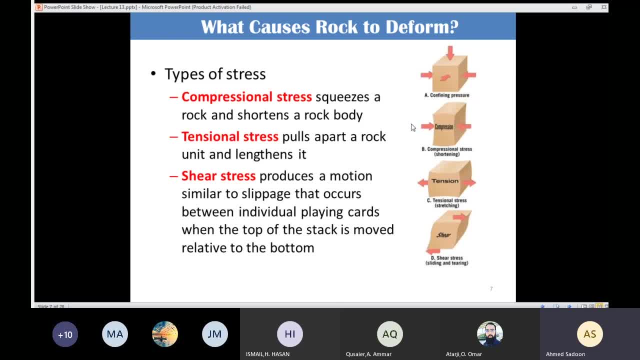 shortens a rock body. this dimension here is going to be shorter than the original length. the other type, which is tensional, uh, compressional stresses. this one is opposite to compressional stress. instead of squeezing something, we are stretching something. we are stretching the rock, or pulls apart a rock until we have increase in the length in that direction here. so the original. 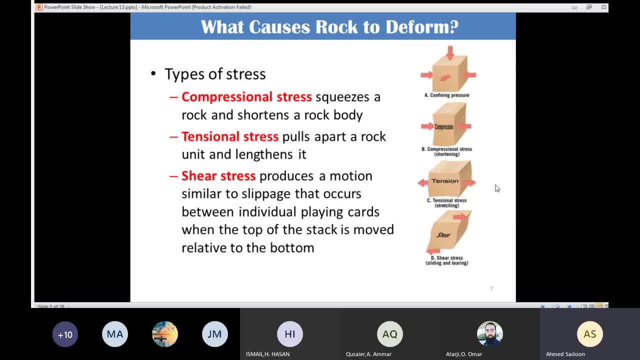 dimension, or the original length, is going to be increased, while in compressional stress the original dimension is going to be decreased. the last one is the shear stress. in this process, we are going to have a motion in a, the top part of the rock, for example. i'm going to fix this part. 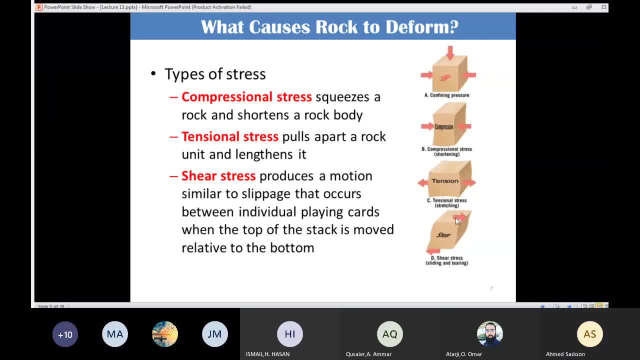 and i'm going to move that part because of the stress here. so we are going to have relative movement. this part is going to move relative to that part. so originally that part, that point it was here and because of that stress at the top of the rock, that point it moved from that point to that. 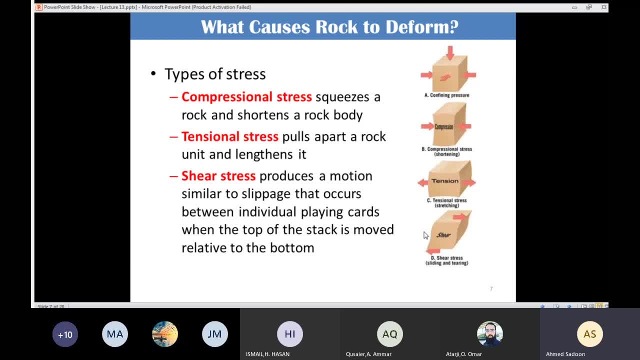 point, and if we are going to have something like that, we are going to call it shear stress. so shear stress reduce a motion similar to slippage that occurs between individual playing cards. when the top of the stack is moved relative to the bottom, it's just like you have the cards you are. 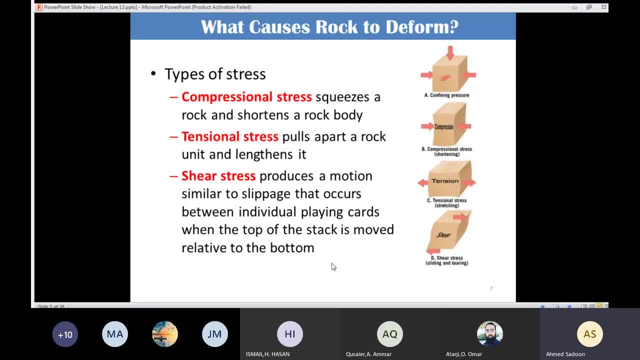 going to move the top card relative to another. in that case we are going to say that we have shear stress. so the differential stress it could be compressional stress, it could be tensional stress, it could be shear stress. if it's compressional stress, that means the original length is going to. 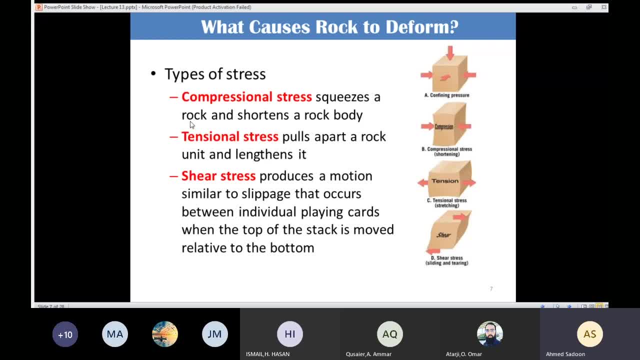 be shorter. if you are going to have tension, tensional stress, in that case we are going. the original length is going to be increased. if i'm going to have shear stress, the top point is going to move relative to another point. any questions so far? any questions so far. 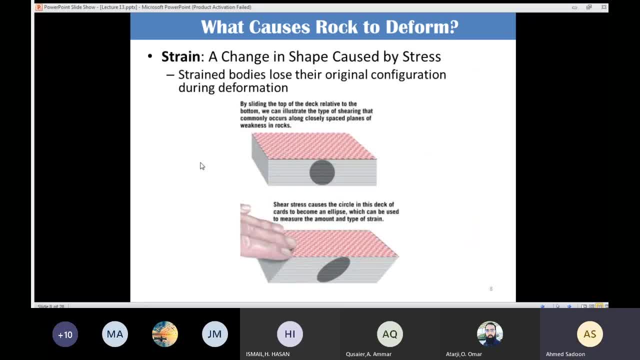 so let's move on. and, as i said, if you have stress, it means that you are going to have strain. so strain means that i have a change in the shape caused by stress. when i have stress, i'm going to have a change in the shape of the rock and we call this strain. so strained bodies lose their original. 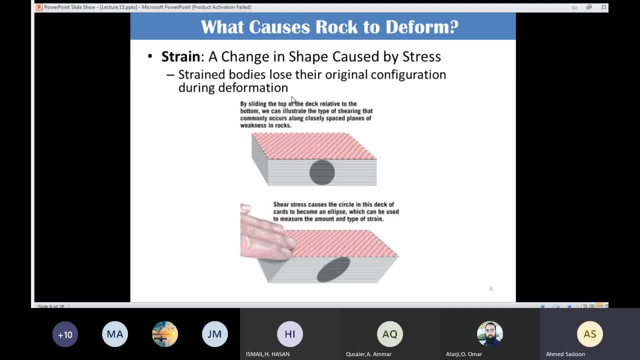 configuration during the formation. so if you apply stress body or to a rock body, we are going to have deformation or a change in a shape. we call it strain. the deformation is a general term. any changes in position in the shape, it's deformation. but strain is a special type of deformation. so if you 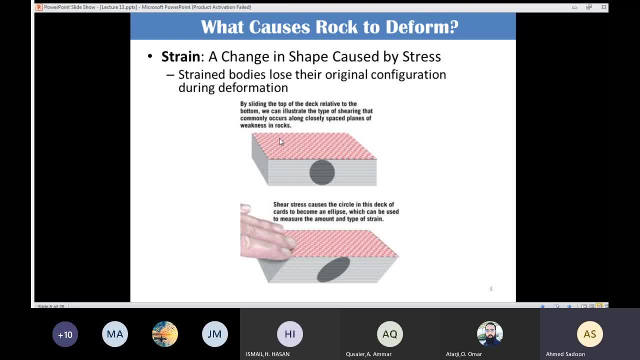 have something like that, and then you are going to apply stress in that service, in other words, I'm going to apply shear stress. so if that service moved relative to that service, the top service moved relative to the bottom service, and assume- here you draw a circle- and if that process took place, 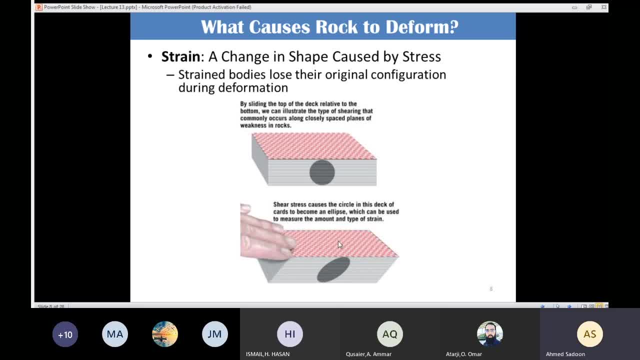 then what happened to a circle here? did you notice the difference between the circle here in the beginning and after the after we apply shear stress? yes, deformation happened. yes, instead of having circle, we have, we are going to have ellipse. so we are going to measure the amount of the strain by how much the circle has been changed. so here is the. 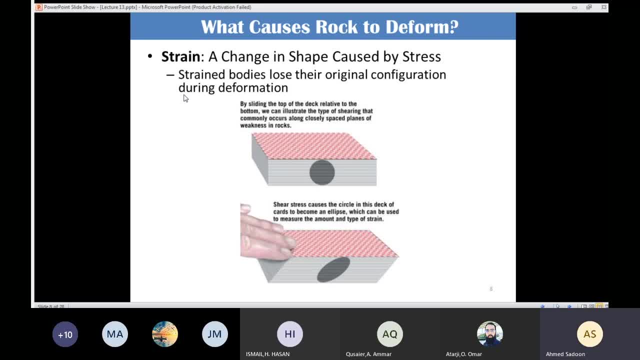 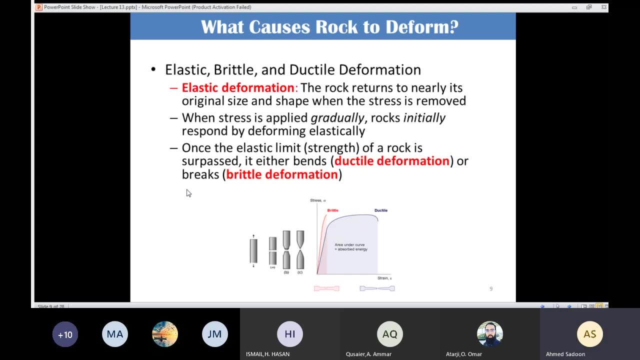 idea of the strain. now we understand what does it mean by stress, what does it mean by strain, and also we learn the confining pressure and the differential stresses. the last point: in order to understand the behavior of the rock, we need to understand the difference between elastic material. 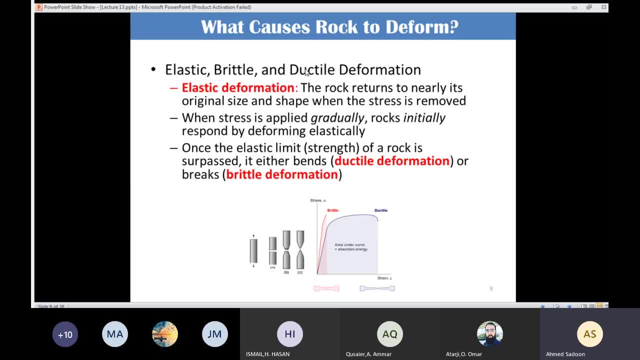 brittle material and the tile deformation or the tile material. so also I know that those who took the strength of material course they are with the concept. but here we are going to explain the concept again so that we can understand the behavior of the rock. so we have elastic deformation, we have 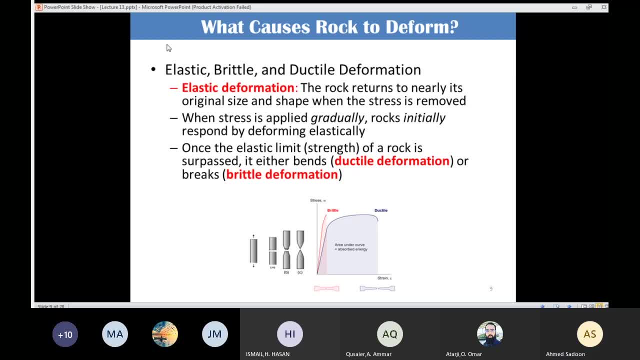 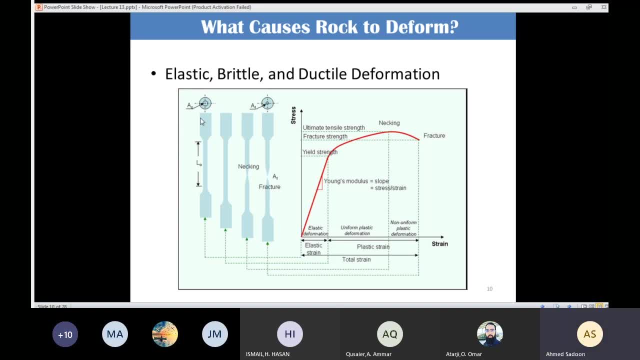 brittle deformation and we have the tile deformation. so to understand this, please look at this picture, or this figure assumes that I have a material and that material is fixed at that part and also it's fixed from that part, and here we have the original length. so the original. 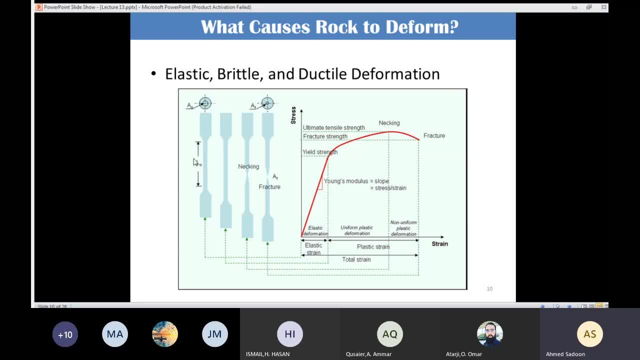 length is going to be referred by the letter L- knot- then I'm going to apply a force, I'm going to stretch that bar here or that road, I'm going to stretch that road from that direction and that direction, which means that I'm going to apply force and this one is going to be fixed and this one is going to be. 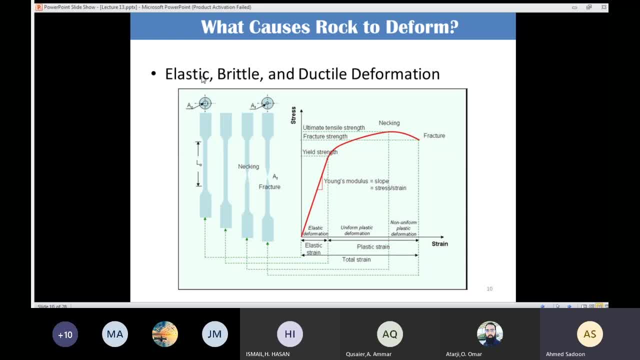 tensional stresses. so, as a result, like I said, when we apply stress, what will happen? we are going to have strain, so the strength is here in a form of increase in the length, so that links in the direction of the force is going to be longer, like you can see here. then I'm going to apply stress, and this one is: 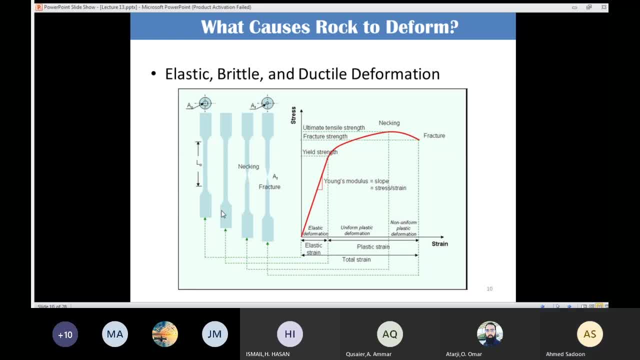 going to bemoding. it is going to be strutting in the direction of the motor guide, so this one is going to be strutting in a direction of the Pasteur wheel and this one is going to be Multi' but it is cutting and this specifically, 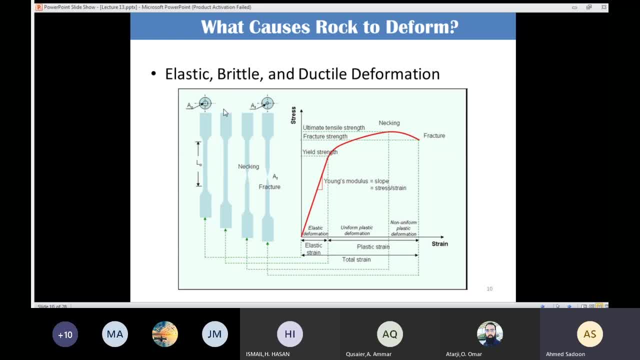 I am going to divide the force with the two lines of the panque to the transverse and transverse six and transverse seven, which means that Sp of L that I have in order to do that. so when I have that stress point I only apply two lines. so that is divided into two lines of the panque. you can have this. 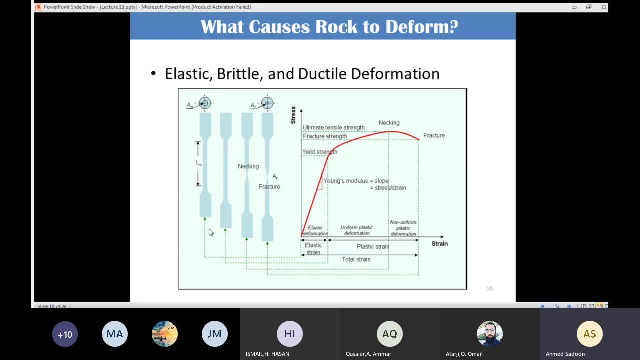 so if I have two lines of the cross section, then what I have over this in the length, if I have increase in the length, it means that I'm going to have a strain. so I have increase in the length. then if I remove that force, what do you? 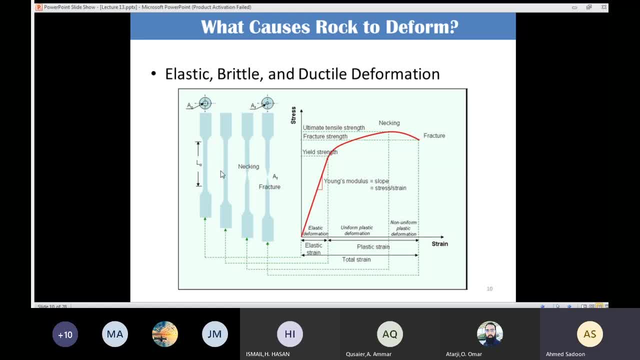 think will happen. I apply a force here and, as a result, I have increase in the length. if I remove this force, in other words, that force here is no longer working on that bar or that rod- what do you think will happen? the material will go back to its original shape. yes, this one possibility, because it is in one. 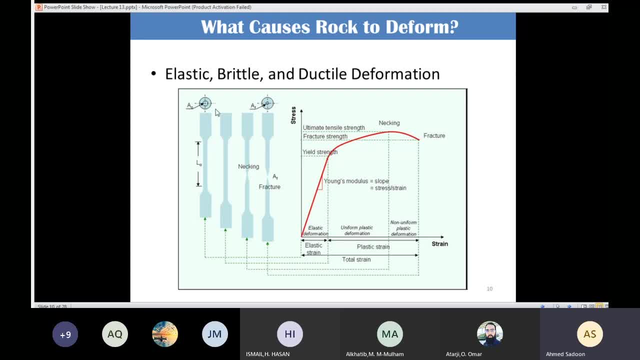 possibility is that the material is going to get to its original shape. so if this one is l1, if this one is l1, the material it may go back to its original length, which is l1, not we could have another possibilities like what the material will stay. 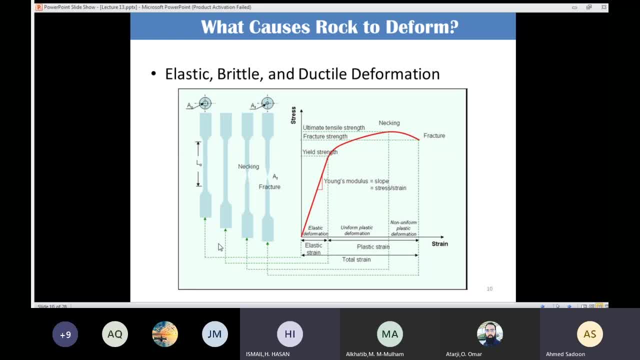 different: deformed. the material could stay deformed. it's the other possibility. so if I stretch a bar, then if I remove the force, I have two possibilities: either to get to its original you length or I could have new links. if I'm going to have new links, that mean I: 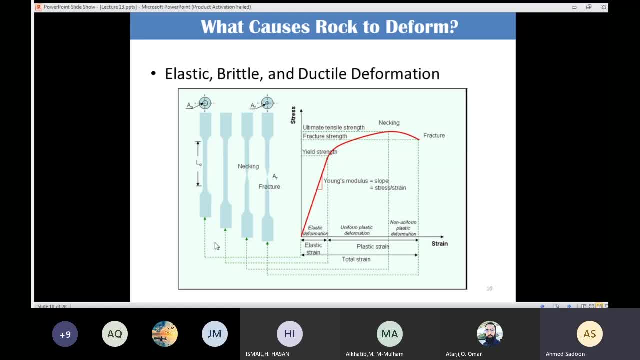 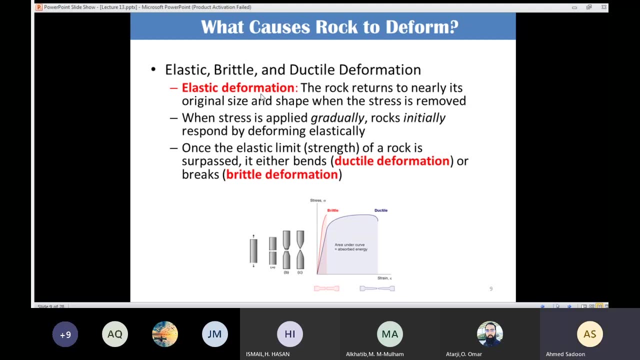 exceed the elastic region. so as long as the material can get back to its original length, we are going to say that we have elastic deformation. so if you apply a stress to a rock and if you release the stress or remove the stress the rock, it will get back to its original shape. in that case we are going to say that we 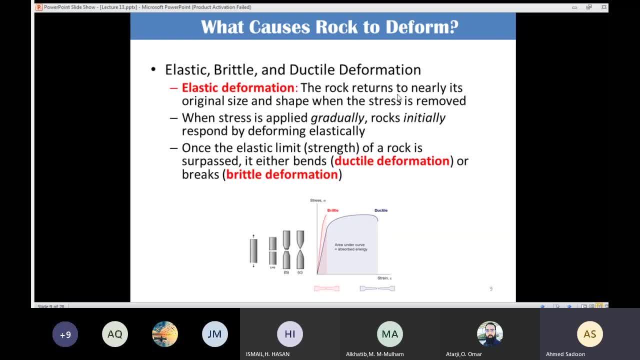 are having elastic deformation, so the rock returns to nearly its original size and shape when the stress is removed. is that point clear for you? any questions about the elastic deformation, isn't it? it's a good question? it's a good question, clear, thank you. so when stress is applied gradually, rocks initially. 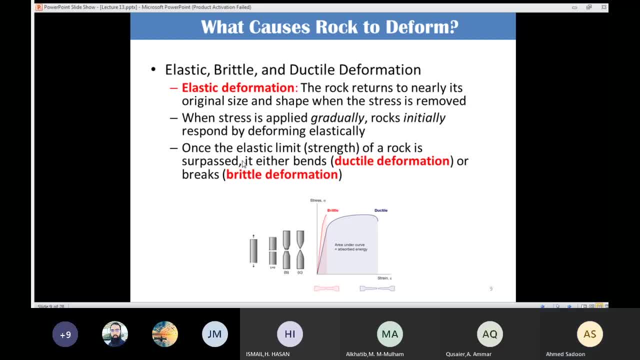 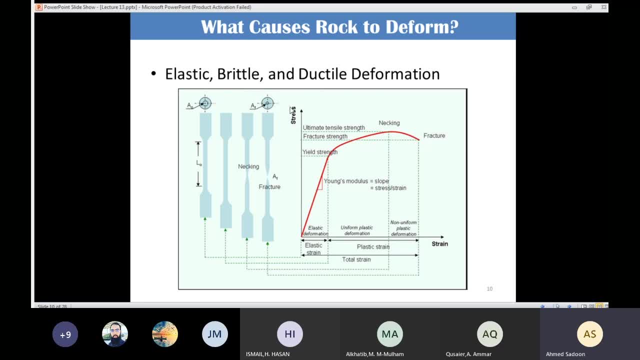 responds by deforming elastically, which means that if I apply the force slowly, start wide by one Newton to Newton, three, four, five. we are going to have gradually response by increasing in the length. if I increase the force then I'm going to have a response by increasing the length and if I remove the for the force of the. 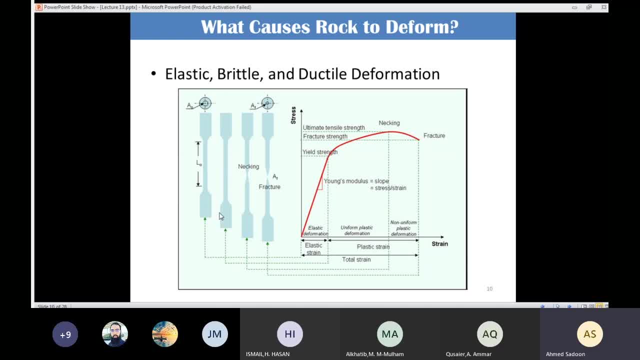 stress at any point if it's get back to its original length, that mean we are still in the elastic region or the elastic deformation. now we are going to look on the other possibility, which is we are going to have permanent deformation, and in order to and that, 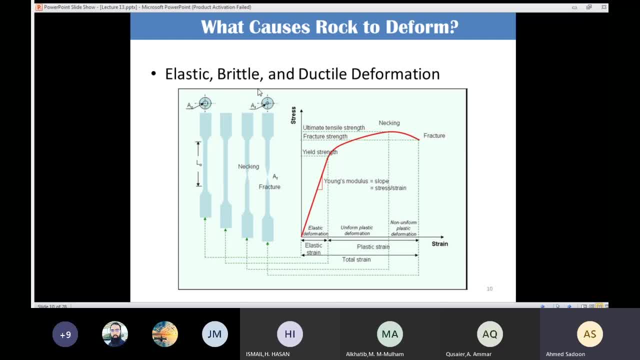 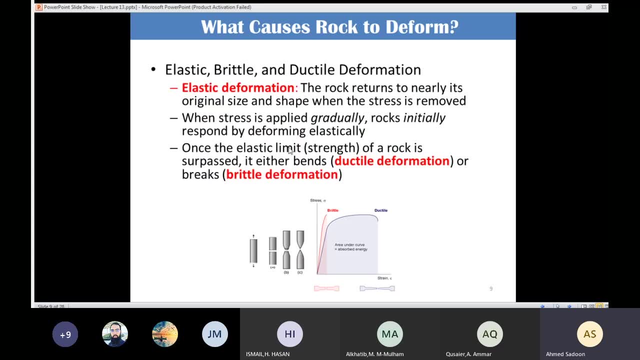 deformation and in order to, and that deformation and in order to, and that depends mainly on the behavior, some depends mainly on the behavior, some depends mainly on the behavior. some material, it has brittle behavior, while material it has brittle behavior, while material it has brittle behavior, while the other it has the file behavior. so 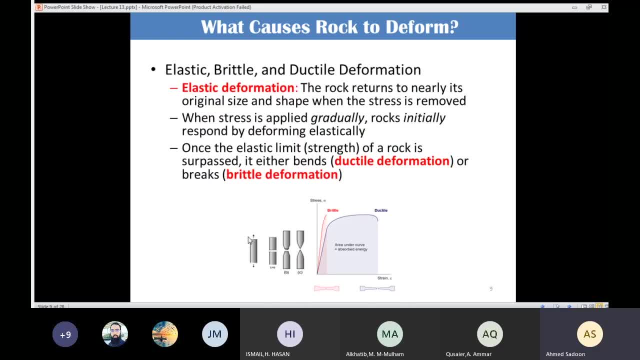 the other it has the file behavior. so the other it has the file behavior. so look at that picture. here we have small. look at that picture. here we have small. look at that picture: here we have small bar and, as you can see, we apply a force bar and, as you can see, we apply a force. 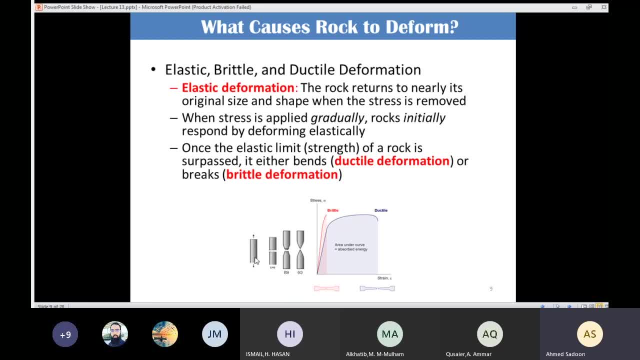 bar and, as you can see, we apply a force and unfortunately, this time we didn't and unfortunately this time we didn't and unfortunately, this time we didn't remove the force. we are going to stretch, remove the force. we are going to stretch, remove the force. we are going to stretch that bar until we catch or reach the. 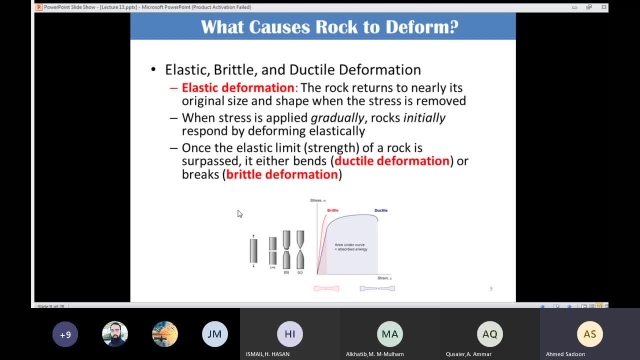 that bar until we catch or reach the, that bar, until we catch or reach the ultimate capacity. we said that each and ultimate capacity. we said that each and ultimate capacity. we said that each and every material, it has a certain level of every material, it has a certain level of. 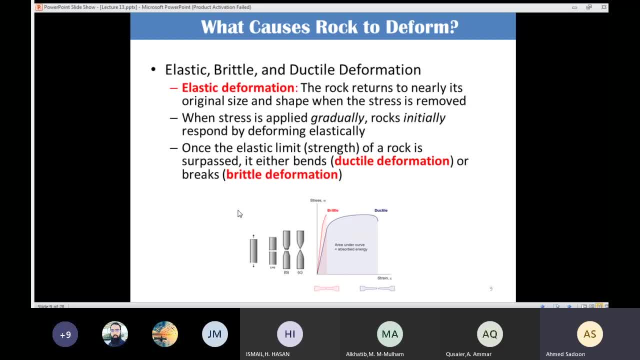 every material, it has a certain level of stress. if you exceed that level of the stress, if you exceed that level of the stress, if you exceed that level of the stress, the failure will take place. so, but stress, the failure will take place. so, but stress, the failure will take place. so, but we have two possibility: the one: 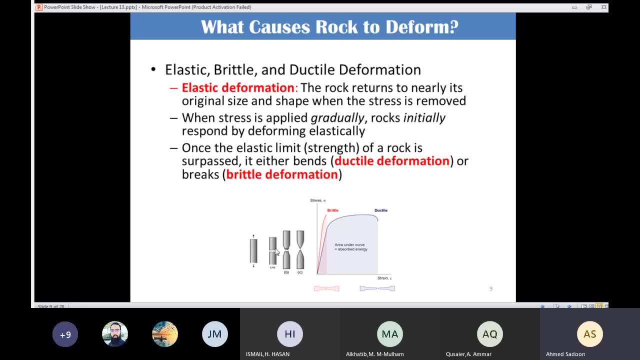 we have two possibility. the one, we have two possibility. the one possibility when you reach the maximum possibility. when you reach the maximum possibility, when you reach the maximum capacity, of course we are going to have capacity, of course we are going to have capacity, of course we are going to have increase in the length, but we are going. 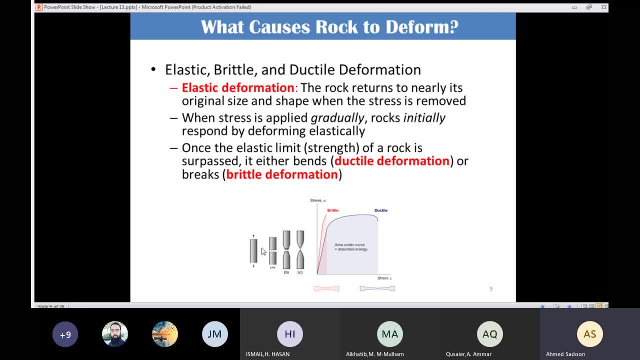 increase in the length, but we are going increase in the length, but we are going to have a sudden failure without any. to have a sudden failure without any. to have a sudden failure without any science like this one, so the material science. like this one, so the material. 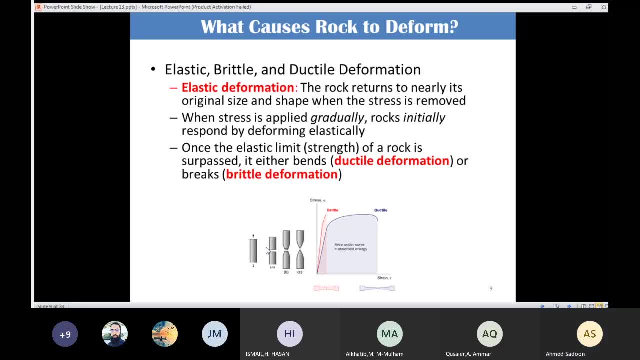 science like this one. so the material here. it didn't show us any science. it's here. it didn't show us any science. it's here. it didn't show us any science. it's just fail. all of sudden, we call this. just fail. all of sudden, we call this. 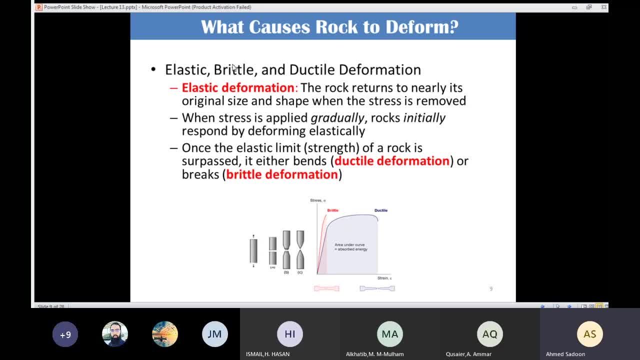 just fail. all of sudden, we call this brittle deformation or brittle behavior. brittle deformation or brittle behavior. brittle deformation or brittle behavior. as a material material could show a sign, as a material material could show a sign, as a material material could show a sign like this one, we call this one necking. 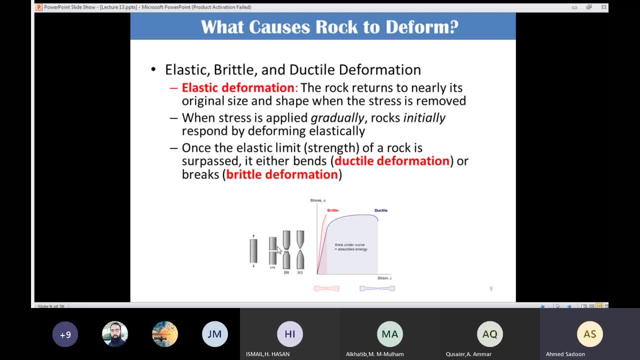 like this one. we call this one necking. like this one. we call this one necking. it will going to show a sign before. it will going to show a sign before. it will going to show a sign before failure, and we are going to call this failure and we are going to call this. 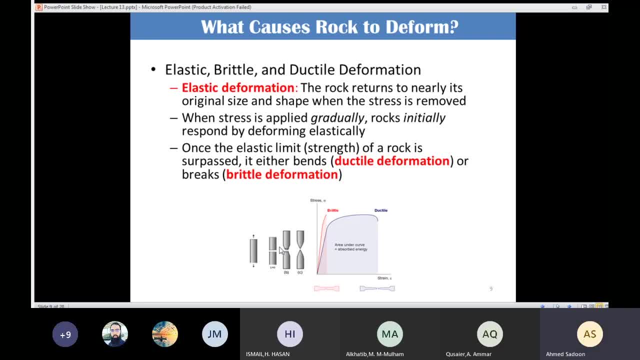 failure, and we are going to call this tactile deformation, the tactile tactile deformation, the tactile tactile deformation, the tactile deformation like you can see before the deformation, like you can see before the deformation, like you can see before the failure, or at the place of the maximum failure, or at the place of the maximum. 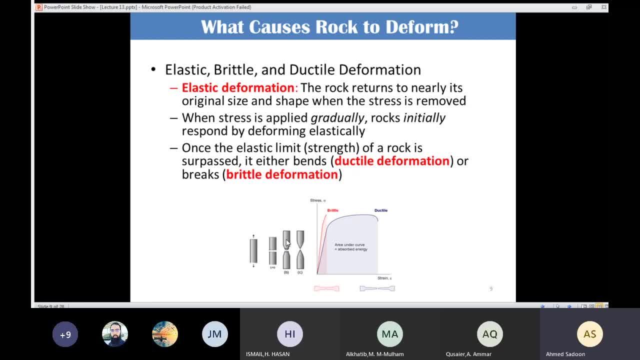 failure, or at the place of the maximum capacity, or the stress we are going to capacity, or the stress we are going to capacity, or the stress we are going to have deformation, large deformation. have deformation, large deformation, have deformation, large deformation. actually compare with the brittle. actually compare with the brittle. 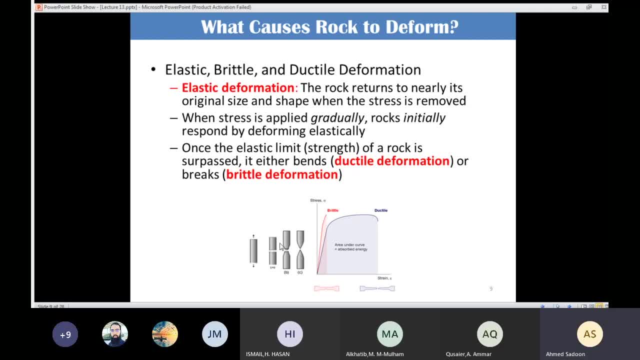 actually compare with the brittle material here before the failure. we are material here before the failure. we are material here before the failure we are going to have going to have going to have necking, necking, necking, necking process like this one before the failure process, like this one before the failure. 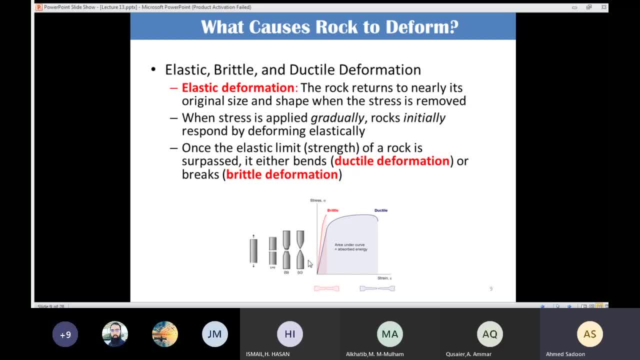 process like this one, before the failure. if you are going to draw the behavior in, if you are going to draw the behavior in, if you are going to draw the behavior in terms of stress and strain are going to terms of stress and strain, are going to terms of stress and strain, are going to draw it or plot it in charts, you are. 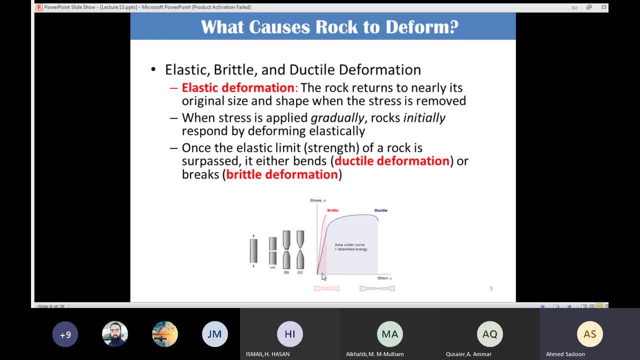 draw it or plot it in charts. you are draw it or plot it in charts. you are going to say that, assume that point is a going to say that. assume that point is a going to say that. assume that point is a point of failure for the brittle. 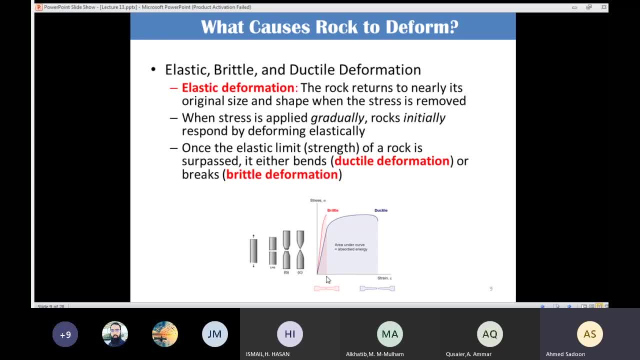 point of failure for the brittle, point of failure for the brittle material when it's get to its maximum material. when it's get to its maximum material, when it's get to its maximum capacity, we are going to have sudden capacity. we are going to have sudden capacity. we are going to have sudden failure like this one. but in case of the 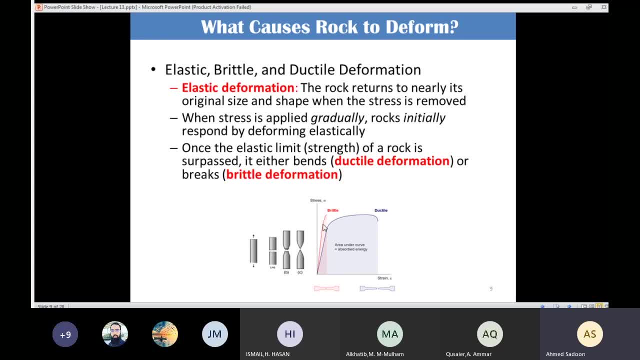 failure like this one. but in case of the failure like this one, but in case of the tile behavior, when the material reach tile behavior, when the material reach tile behavior, when the material reach its maximum capacity, you are going to its maximum capacity. you are going to its maximum capacity. you are going to have large deformation compared with the 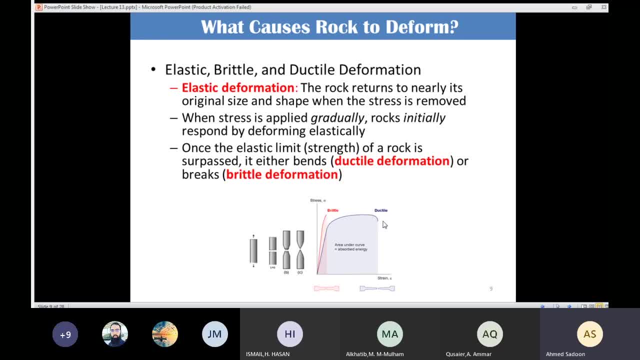 have large deformation compared with the have large deformation compared with the stress with a small stress. we are going stress with a small stress. we are going stress with a small stress. we are going to have large deformation and this one to have large deformation and this one to have large deformation and this one is is illustrated by that neck in here. so 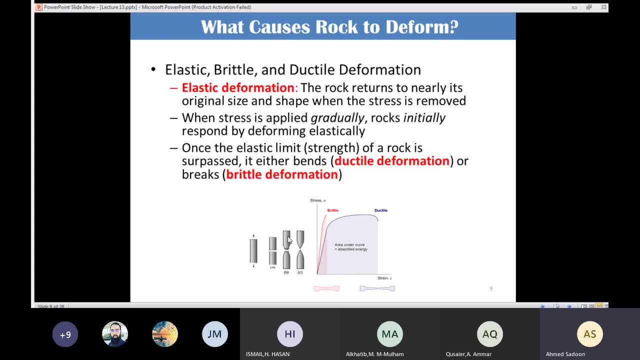 is illustrated by that neck in here. so is illustrated by that neck in here. so if I'm going to have large deformation, if I'm going to have large deformation, if I'm going to have large deformation compared with the stresses after the, compared with the stresses after the. 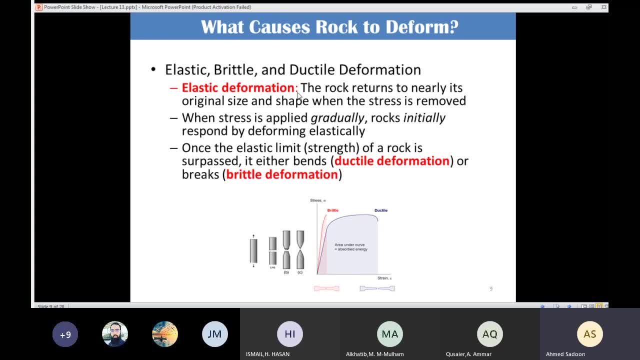 compared with the stresses after the material reaches maximum capacity. we are. material reaches maximum capacity. we are. material reaches maximum capacity. we are going to say that. we are going to have going to say that we are going to have going to say that we are going to have the tile deformation. and if you have 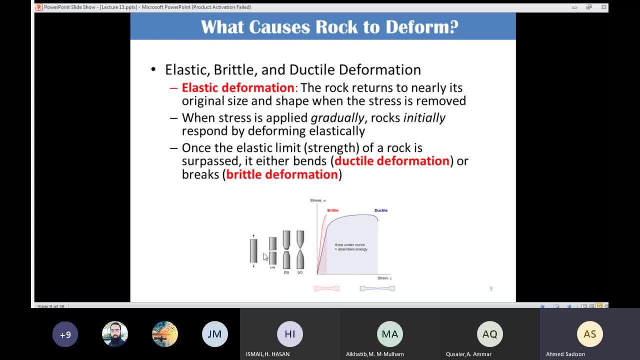 the tile deformation. and if you have the tile deformation, and if you have sudden failure like this one, without sudden failure like this one, without sudden failure like this one, without showing large deformation before failure, showing large deformation before failure, showing large deformation before failure, we are going to say that we, we are. 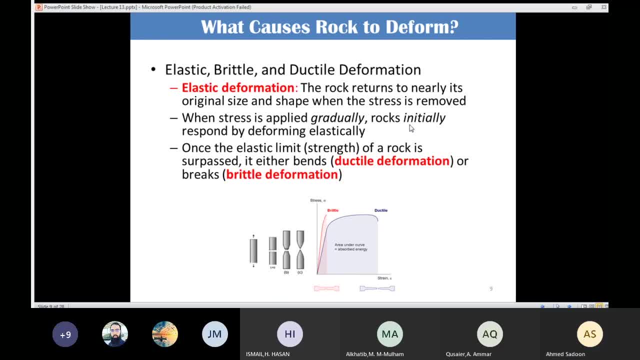 we are going to say that we, we are. we are going to say that we, we are having brittle deformation. so once the having brittle deformation, so once the having brittle deformation, so once the elastic limit strings of the rock is elastic, limit strings of the rock is elastic, limit strings of the rock is suppressed. it's either bends which mean 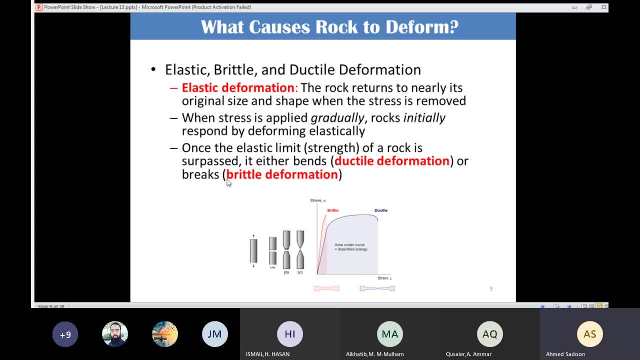 suppressed. it's either bends which mean suppressed. it's either bends which mean that the tile deformation, or bricks like that, the tile deformation, or bricks like that the tile deformation, or bricks like the brittle deformation with the bricks, the brittle deformation with the bricks, the brittle deformation with the bricks like this one, or bent like that one. 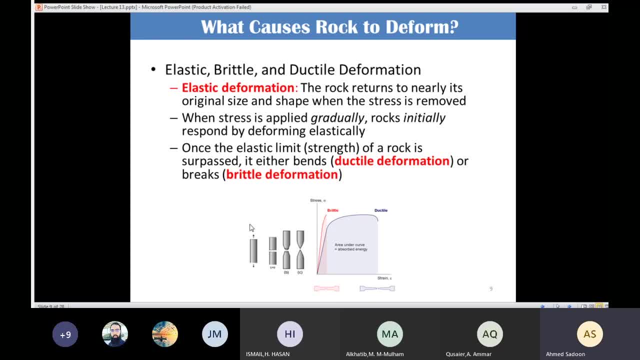 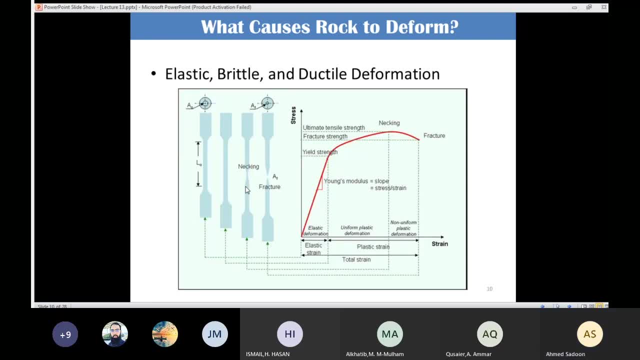 like this one, or bent like that one, like this one or bent like that one, showing necking. so after the elastic showing necking, so after the elastic showing necking, so after the elastic limit, either to have the tile limit, either to have the tile limit, either to have the tile deformation or brittle deformation. so 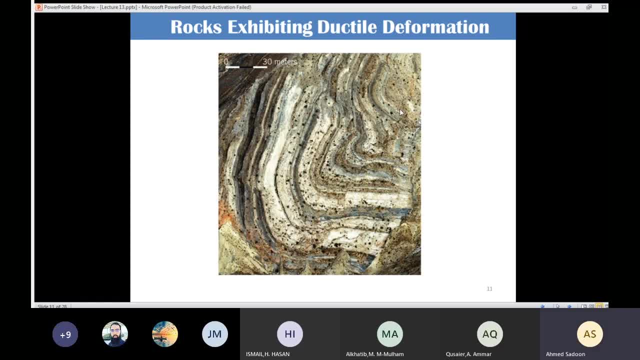 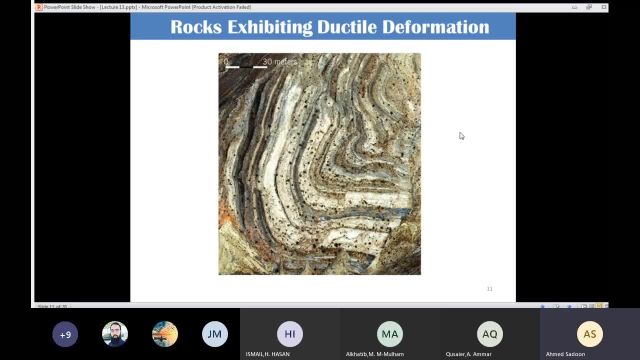 like you can see, you have deformation right. so how we are going to classify that? so how we are going to classify that. so how we are going to classify that deformation: is it the tile deformation or deformation? is it the tile deformation or deformation? is it the tile deformation or brittle deformation? and why this is the. 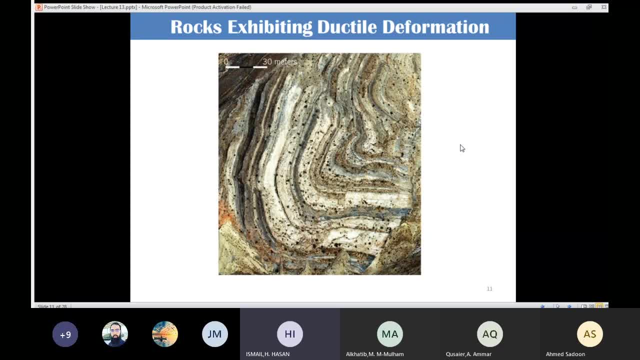 brittle deformation and why this is the brittle deformation and why this is the image. image across section area- cross image. image across section area- cross image. image across section area- cross section image. this image here: it show us section image. this image here: it show us section image. this image here: it show us the structure, the inside structure of the. 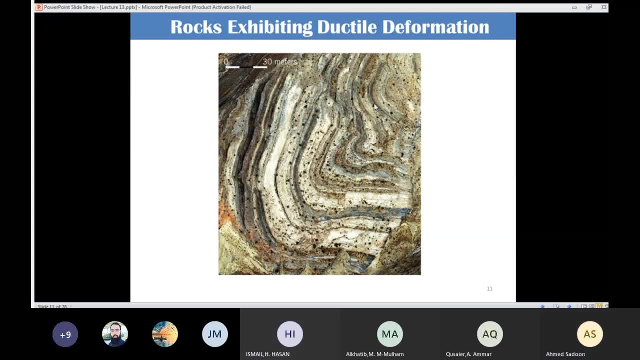 the structure, the inside structure of the. the structure, the inside structure of the rock: okay, rock, okay, rock, okay, so it's obviously the rock is was so it's obviously the rock is was, so it's obviously the rock is. was subjected to stresses and, as a result, we 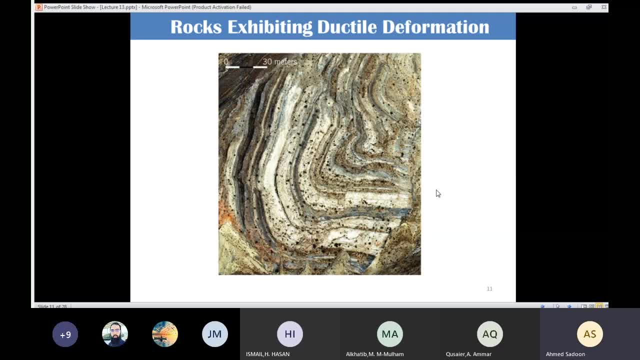 subjected to stresses and, as a result, we subjected to stresses and, as a result, we have deformation inside the rock. so have deformation inside the rock. so have deformation inside the rock. so which one, which one is this type of which one? which one is this type of which one? which one is this type of deformation? is it the tile or is it? 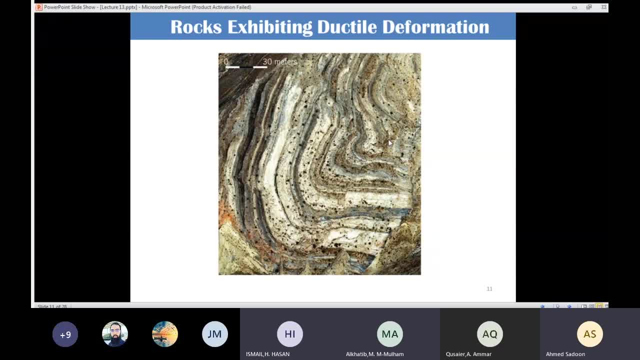 deformation. is it the tile or is it deformation? is it the tile or is it brittle and why? my guess is the time why brittle and why? my guess is the time why brittle and why? my guess is the time why. you sorry, it's good guess, but why? 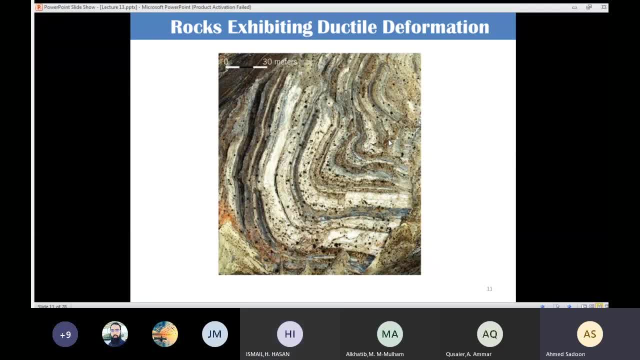 you sorry, it's good guess, but why you sorry it's good guess, but why? because the curved line break line. it's because the curved line break line, it's because the curved line break line, it's all curved line, all curved line, all curved line. yes, it means that i have bending right. 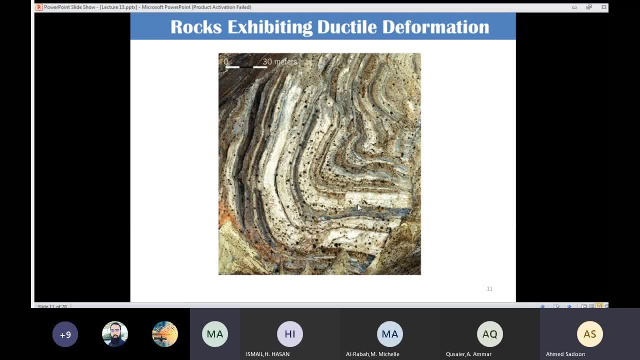 yes, it means that i have bending right. yes, it means that i have bending right. i have necking process here. i have necking process here. i have necking process here. if it's ductile, what do you think will? if it's ductile, what do you think will? 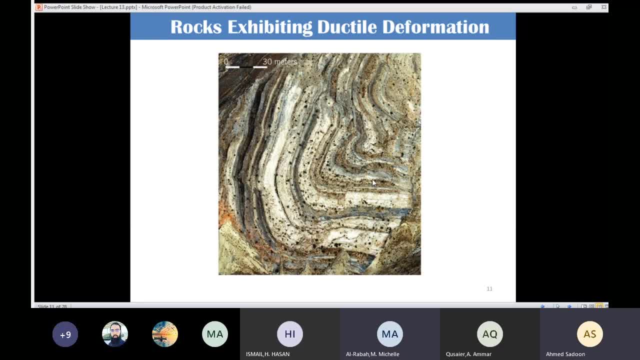 if it's ductile, what do you think will happen? happen, happen, there will be breaks line. yes, i'm going there will be breaks line. yes, i'm going there will be breaks line. yes, i'm going to have to have to have. i'm going to have fractures instead of 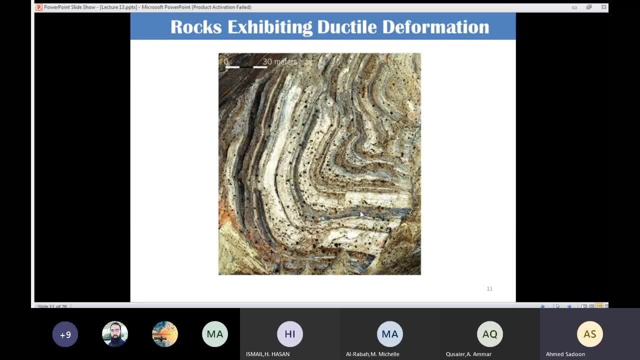 i'm going to have fractures instead of. i'm going to have fractures instead of having having having bending like this one, because the material bending like this one, because the material bending like this one, because the material it doesn't have the capacity to bend. it doesn't have the capacity to bend. 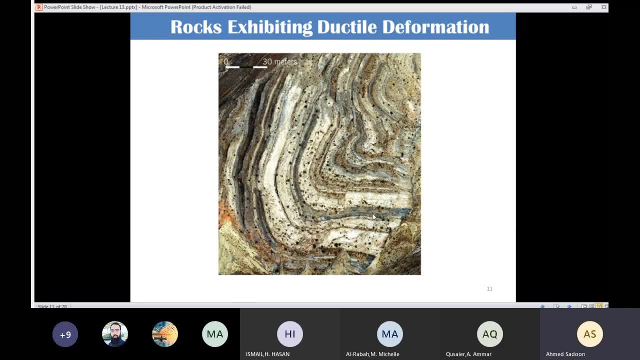 it doesn't have the capacity to bend. so it's good you understand the the. so it's good you understand the the. so it's good you understand the the pile deformation and the brittle pile deformation and the brittle pile deformation and the brittle deformation, deformation, deformation. so before i move to the last point, 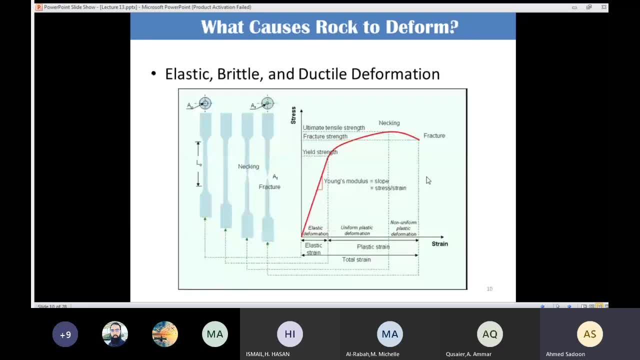 so before i move to the last point, so before i move to the last point here today, here today, here today, do you have any questions about the? do you have any questions about the? do you have any questions about the? the difference between elastic, the difference between elastic. 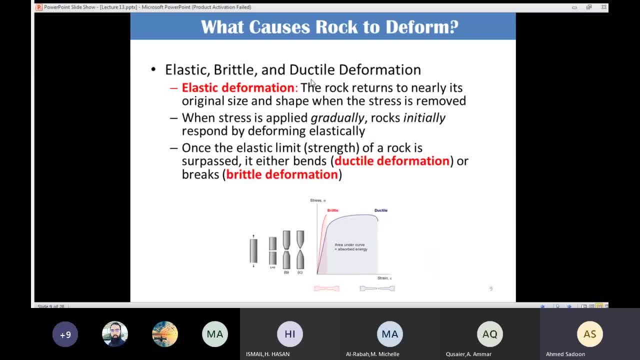 the difference between elastic behavior, brittle behavior and the tile behavior, brittle behavior and the tile behavior, brittle behavior and the tile tactile behavior. does it make sense for all of you? does it make sense for all of you? does it make sense for all of you? i have a question. 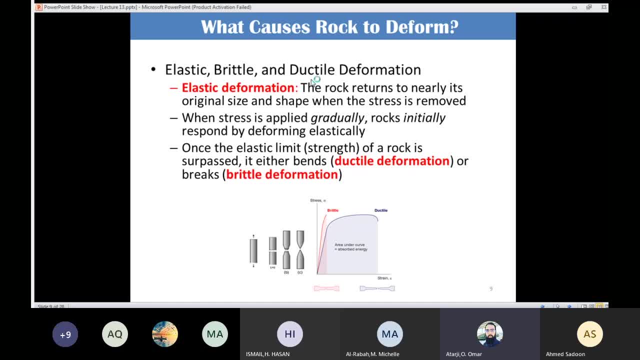 i have a question, i have a question. yes, yes, please. usually we deal with uh i. yes, yes, please. usually we deal with uh i. yes, yes, please. usually we deal with uh i remember, remember, remember, visually we deal with ductile and visually we deal with ductile and. 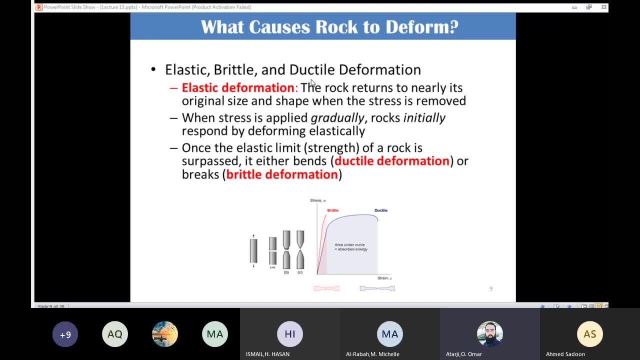 visually, we deal with ductile and brittle, with the brittle, with the brittle, with the tensile stress, but do we apply the same tensile stress? but do we apply the same tensile stress? but do we apply the same concept for compression stress, concept for compression stress. 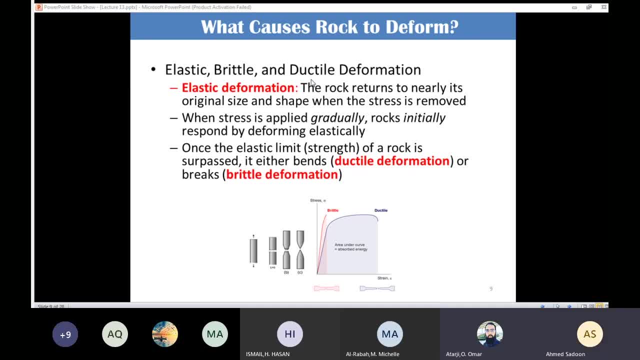 concept for compression stress, applying the, applying the, applying the compressional stress. we're going to see compressional stress. we're going to see compressional stress. we're going to see this in the next section, this in the next section, this in the next section. here we are going to. 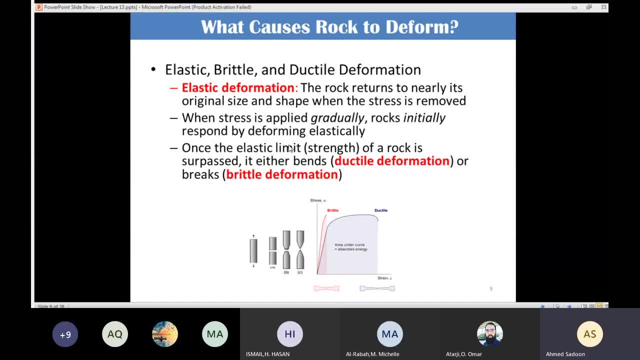 here we are going to, here we are going to see the uh. if we have compressional, see the uh. if we have compressional, see the uh. if we have compressional stress, stress, stress and tensional stress and also sheer and tensional stress and also sheer. 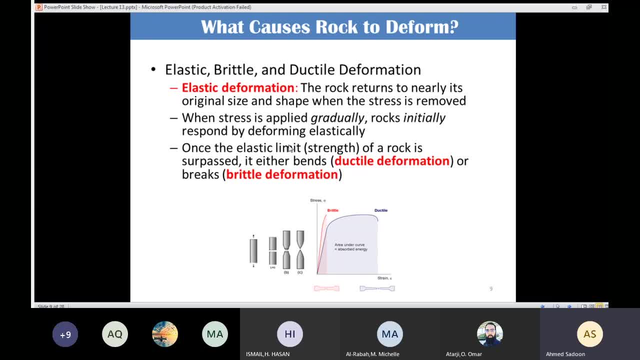 and tensional stress and also sheer stress, stress, stress, and i'm going also, i'm going, we are, and i'm going also, i'm going, we are, and i'm going also, i'm going, we are going to say, going to say, going to say, when we have brittle behavior, what will? 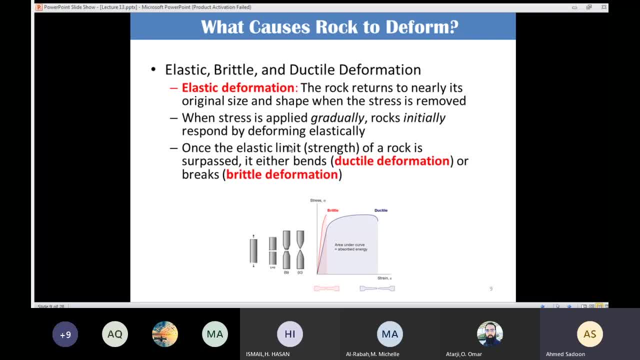 when we have brittle behavior. what will? when we have brittle behavior, what will happen? happen, happen. and if we have uh, if we have the tile and if we have uh, if we have the tile and if we have, uh, if we have the tile, behavior, behavior, behavior- then what will happen? i'm going to go. 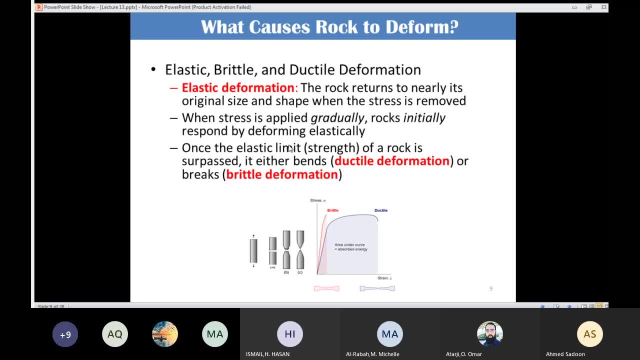 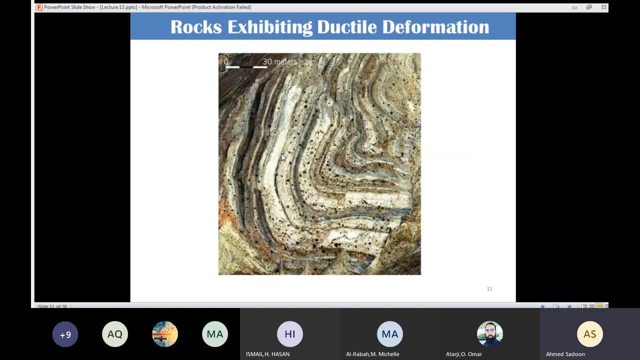 then what will happen? i'm going to go then. what will happen? i'm going to go through that, through that, through that. okay. any other questions regarding the? any other questions regarding the. any other questions regarding the elastic brittle and the tile behavior. so let's move on. 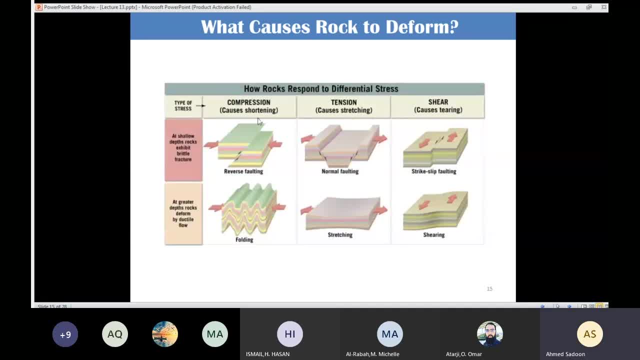 so let's move on, so, let's move on. so i was talking about this, so i was talking about this, so i was talking about this. here, here, here, so, so, so. here in that row, we are going to say the. here in that row, we are going to say the. 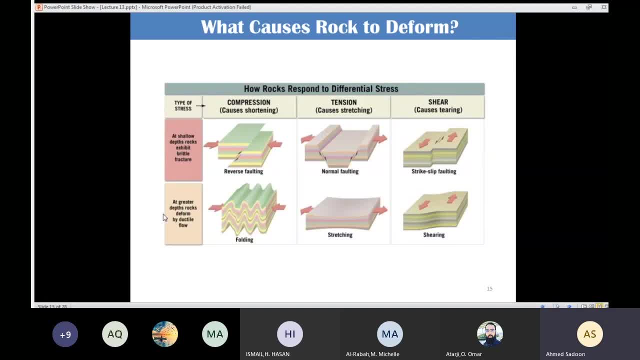 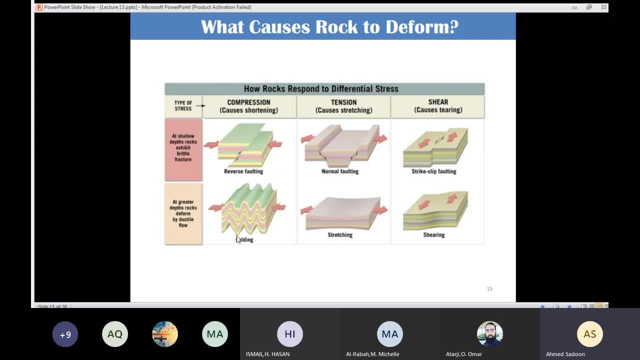 the. the behavior. the- the behavior is tactile, is tactile, is tactile. in that column we are going to say the. in that column we are going to say the. in that column we are going to say: the rock is going to be subjected to, rock is going to be subjected to. 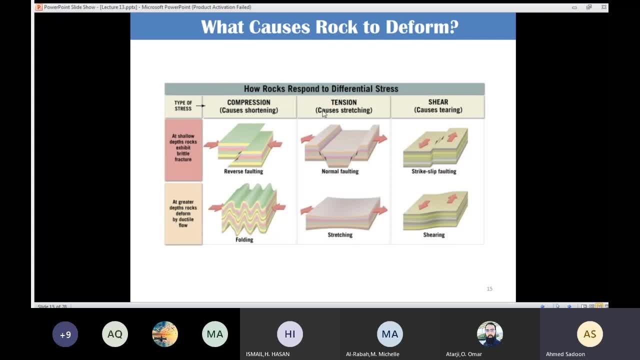 rock is going to be subjected to compressional stress in that column. the compressional stress in that column, the compressional stress in that column the rock is going to be subjected to. rock is going to be subjected to. rock is going to be subjected to tensional stress. 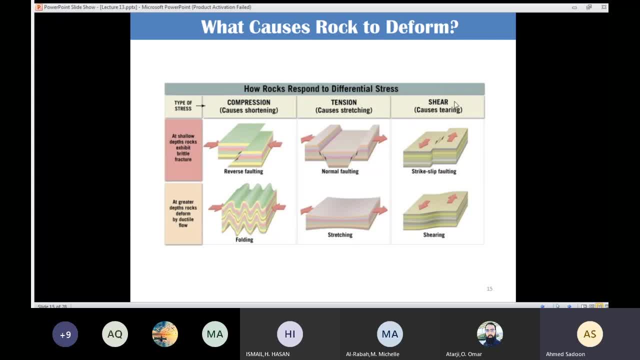 tensional stress, tensional stress, and in that column the rock is going to and in that column the rock is going to, and in that column the rock is going to be subjected to sheer be subjected to, sheer be subjected to sheer stress. so, stress, so, stress. so, as you can see here, 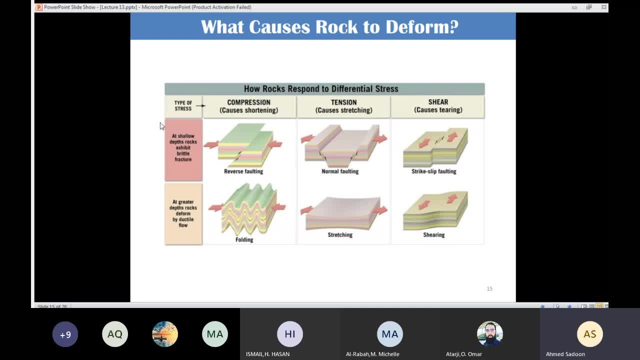 as you can see here, as you can see here, compressional stress. in that case we are compressional stress. in that case we are compressional stress. in that case we are going to have a brick going to have a brick going to have a brick or fracture like this one with relative. 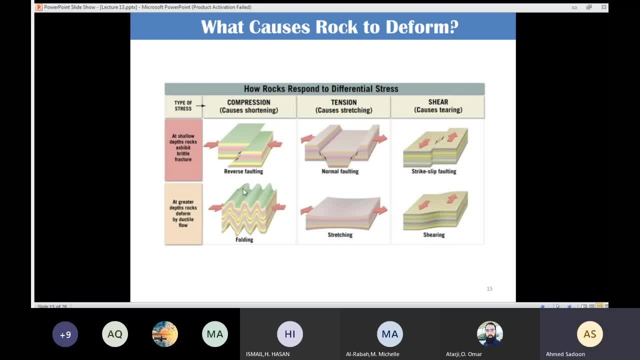 or fracture like this one with relative, or fracture like this one with relative movement, movement, movement. and if the material, and if the material and if the material was, was, was ductile, ductile. ductile if it's subjected to compressional, if it's subjected to compressional. 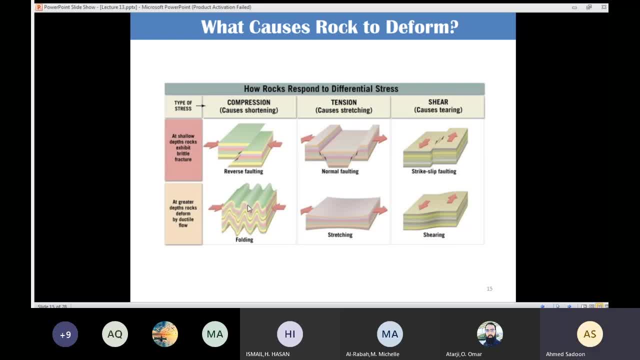 if it's subjected to compressional stress, then i'm going to have stress, then i'm going to have stress, then i'm going to have folding, which means that folding, which means that folding, which means that we are going to have bending like this. we are going to have bending like this. 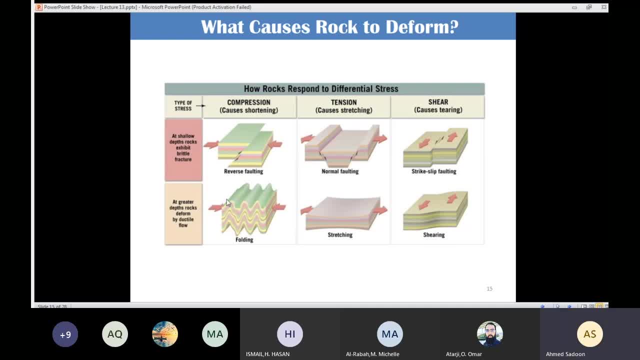 we are going to have bending like this, one one, one in shape of waves, then in shape of waves, then in shape of waves, then if the rock is subjected to tensional, if the rock is subjected to tensional, if the rock is subjected to tensional stresses, if it's brittle, 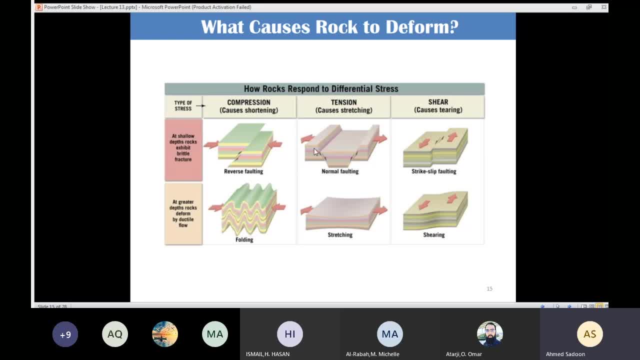 stresses if it's brittle stresses. if it's brittle, then also i'm going to have fracture like. then also i'm going to have fracture like. then also i'm going to have fracture like this one, this one, this one with relative movement, with relative movement, with relative movement, if it's ductile, then i'm going to have. 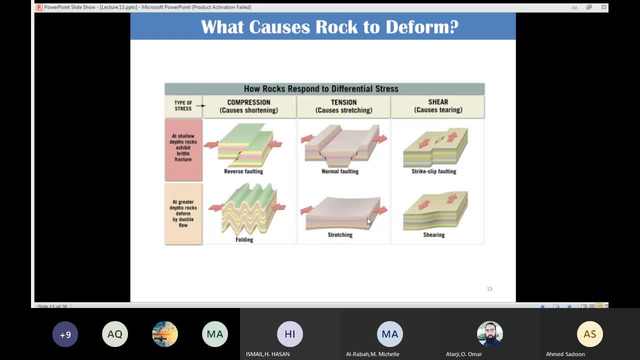 if it's ductile, then i'm going to have. if it's ductile, then i'm going to have stretching like this one. did you understand my the idea here? did you understand my the idea here? did you understand my the idea here? did i answer your question? 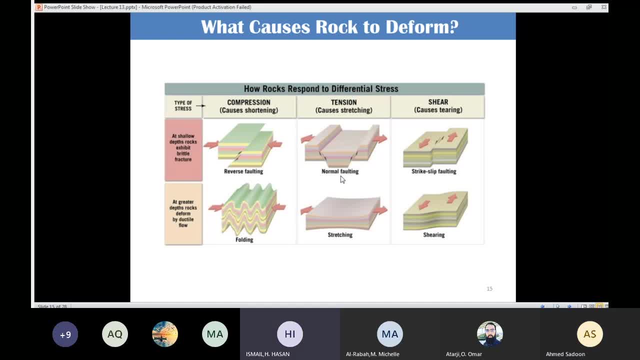 did i answer your question? did i answer your question? uh, doctor, i have another question, if i may, uh doctor, i have another question, if i may. uh doctor, i have another question, if i may. so i answer question, then i get other. so i answer question, then i get other. 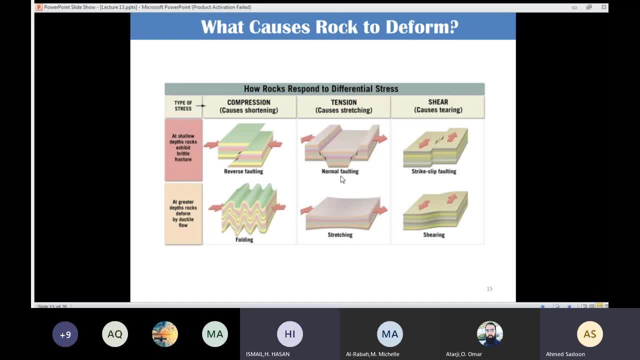 so i answer question, then i get other question. good question, good question. good, okay, give me my guess. okay, give me my guess. okay, give me my guess. uh, doctor, our understanding of rocks. uh, doctor, our understanding of rocks. uh, doctor, our understanding of rocks, that they are brittle material. 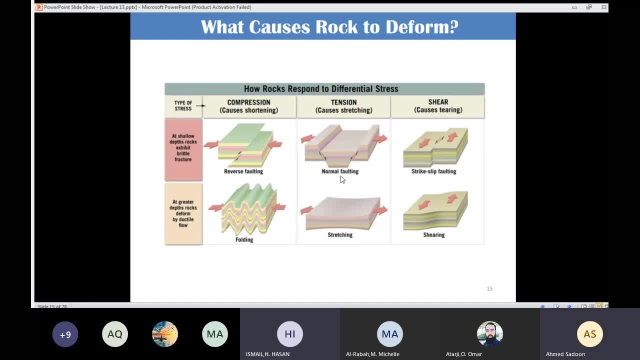 that they are brittle material, that they are brittle material. how can rocks be ductile? how can rocks be ductile? how can rocks be ductile? no, no, also, i'm going to go through that. no, no, also i'm going to go through that. no, no, also i'm going to go through that point. 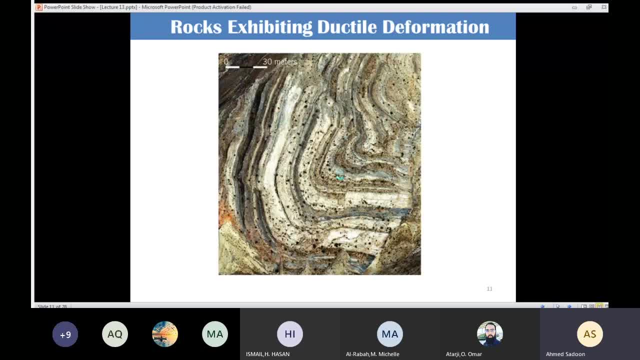 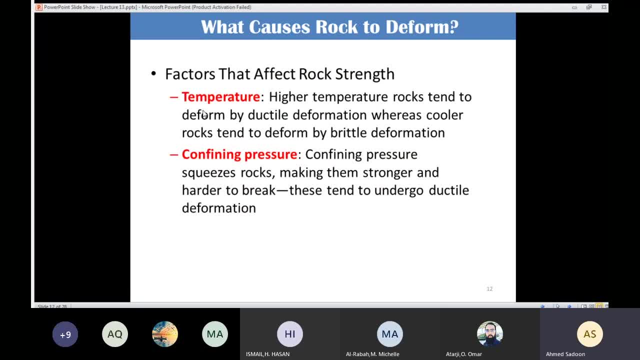 first, the factor is temperature. if i'm going to have higher temperature, if i'm going to have higher temperature, if i'm going to have higher temperature, the rocks tend to deform by the tile. the rocks tend to deform by the tile. the rocks tend to deform by the tile: deformation. 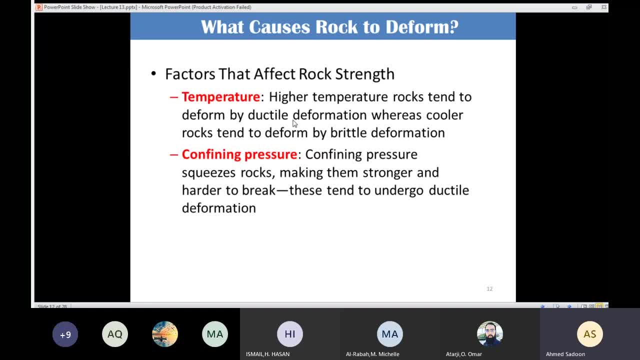 if you are having lower temperature. if you are having lower temperature, if you are having lower temperature, the rocks tend to deform by brittle. the rocks tend to deform by brittle. the rocks tend to deform by brittle. deformation, deformation, deformation also. if you are, if your rock is also, if you are, if your rock is. 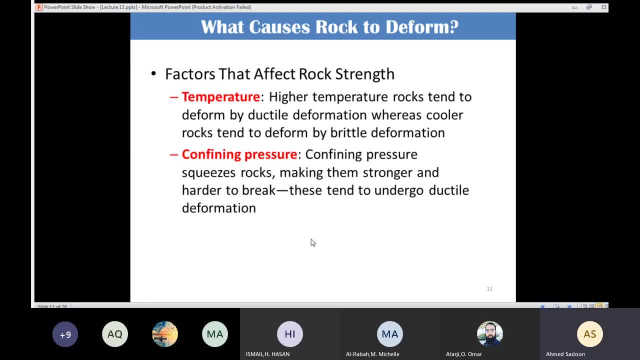 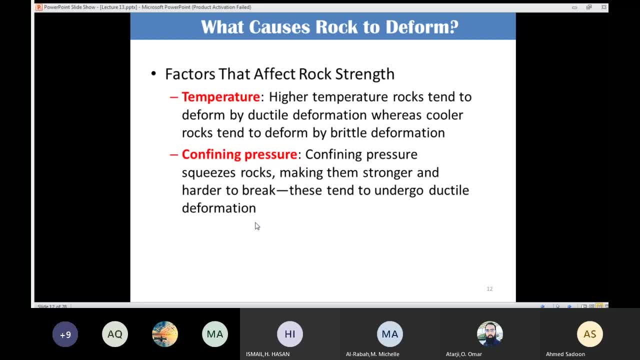 the rock we're going to tend, or the deform, deform, deform by the ductile deformation. i have other by the ductile deformation. i have other by the ductile deformation. i have other factors, factors, factors. the rock type itself if it's made from, the rock type itself if it's made from. 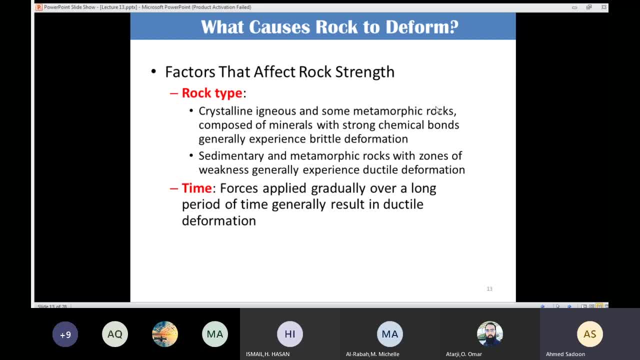 the rock type itself, if it's made from igneous rock. igneous rock, igneous rock and some kind of metamorphic rock, the and some kind of metamorphic rock, the and some kind of metamorphic rock, the. the behavior tend to be brittle. the behavior tend to be brittle. 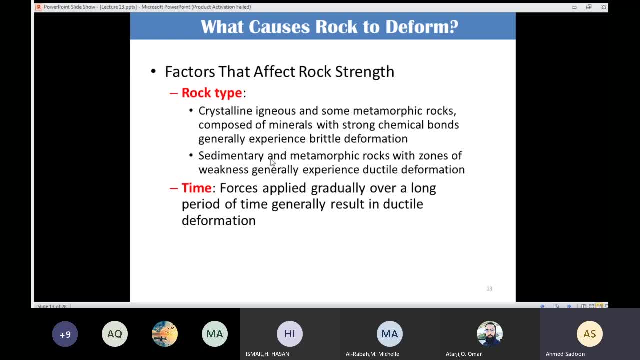 the behavior tend to be brittle. and if it's made from sedimentary, and if it's made from sedimentary, and if it's made from sedimentary and some kind of metamorphic rocks, the and some kind of metamorphic rocks, the and some kind of metamorphic rocks, the behavior is going to be ductile. 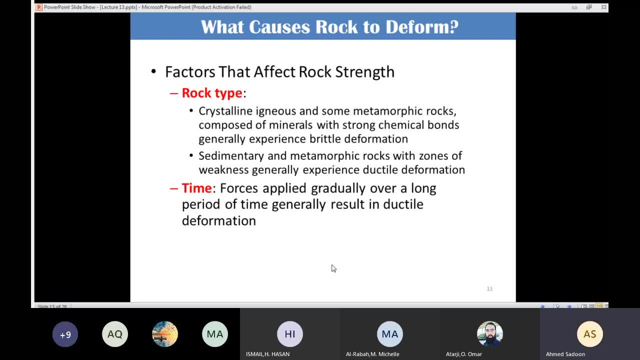 behavior is going to be ductile behavior is going to be ductile deformation, deformation, deformation also. we have another factors for that, we also. we have another factors for that, we also. we have another factors for that. we have the time itself, have the time itself, have the time itself, forces applied gradually over a long 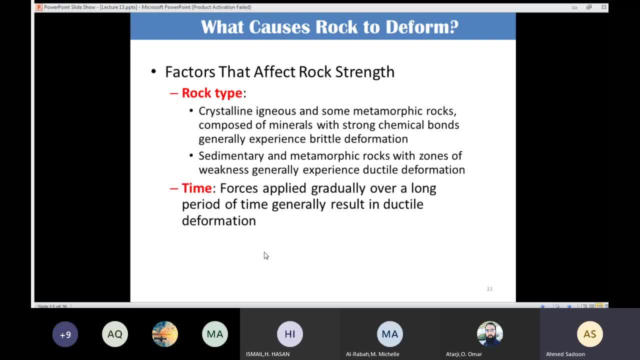 forces applied gradually over a long forces applied gradually over a long period of time, period of time, period of time generally result in ductile deformation. did i answer your question? did i answer your question? did i answer your question? yes, yes, yes, so so so i'm happy that you ask question. 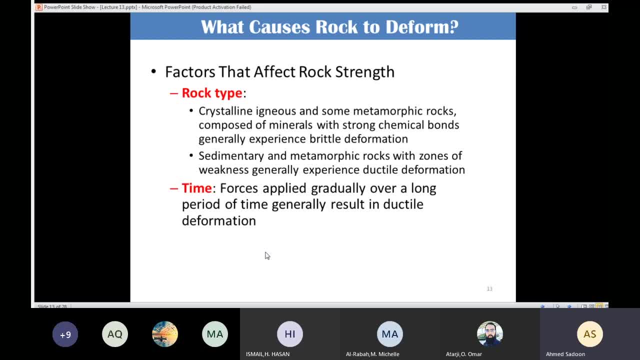 i'm happy that you ask question. i'm happy that you ask question and, and, and. already you are going to the, the, the. already you are going to the, the, the. already you are going to the, the, the. cover that. points which mean that you cover that. points which mean that you. 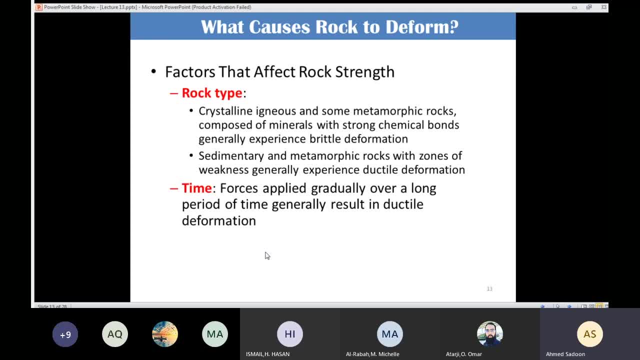 cover that points which mean that you are following the lecture. you are are following the lecture. you are are following the lecture. you are enjoying the lecture, which make me very enjoying the lecture, which make me very enjoying the lecture, which make me very happy, happy, happy. okay, i'm going to stop here. 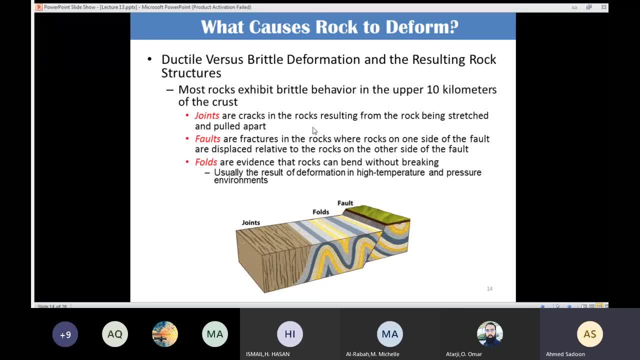 okay, i'm going to stop here. okay, i'm going to stop here. next time we are going to discuss, next time we are going to discuss. next time we are going to discuss the uh different type of deformation, like the uh different type of deformation, like the uh different type of deformation like the joints, faults, flats. 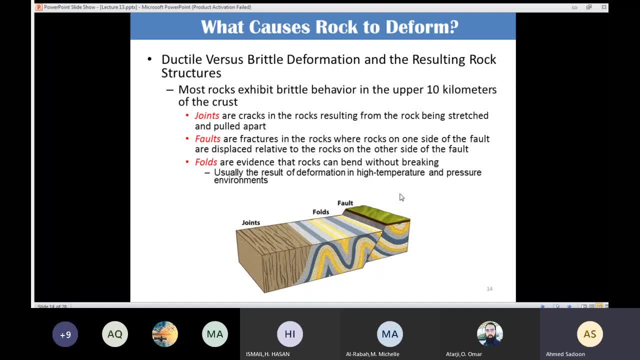 the joints, faults, flats, the joints, faults, flats, and we are going to have more different and we are going to have more different and we are going to have more different information and more, more information about the uh, this type of more information about the uh, this type of. 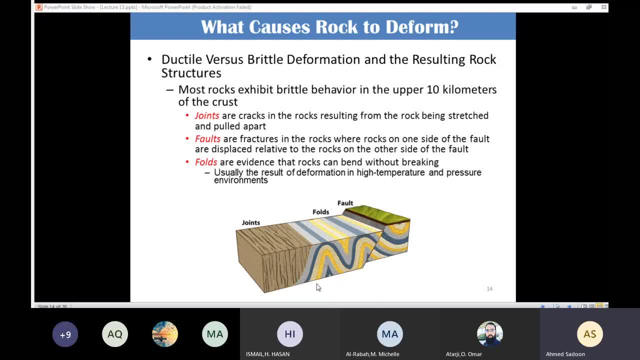 more information about the uh, this type of the deformation, the deformation, the deformation. okay, i'm going to stop here next time. okay, i'm going to stop here next time. okay, i'm going to stop here next time we are going. i'm going to pick up from: 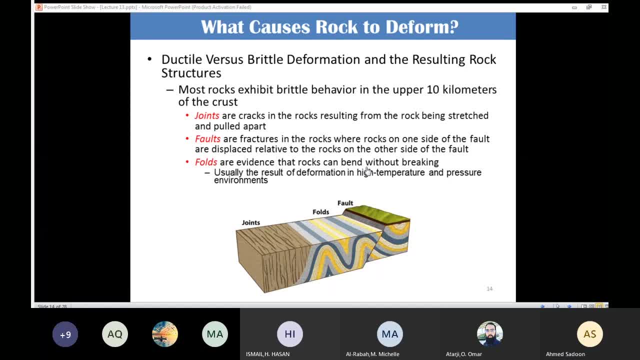 we are going, i'm going to pick up from. we are going, i'm going to pick up from here, here, here. any other questions? 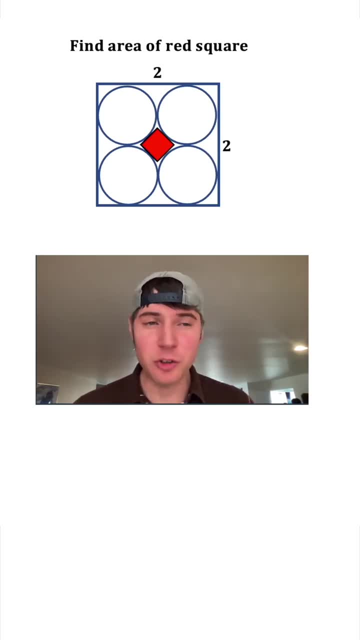 Hey guys, here's another geometry challenge. We have a square that's a two by two square. I have four circles stuck inside of that square and there's another square turned 45 degrees and fit inside those circles so that it touches at those four points, And we want to know what is. 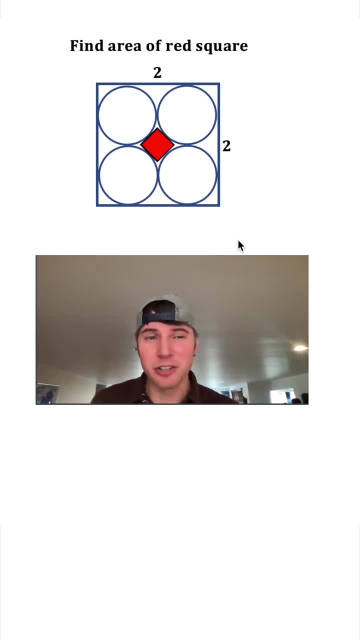 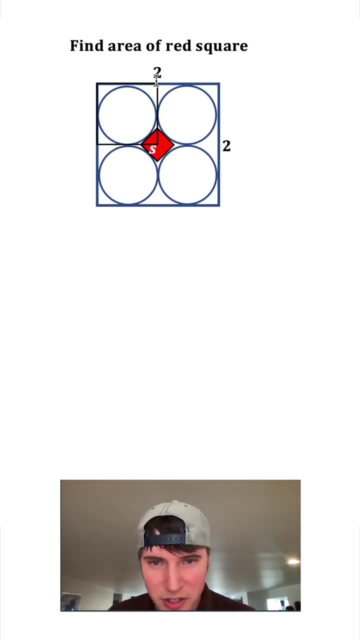 the area of this square. I think there's two ways to solve this. I kind of want to show you both ways. We'll call one side of the square a length of S- S for side or square. Then we'll draw a little square here and we'll notice that this square right here cuts into exactly one. fourth: 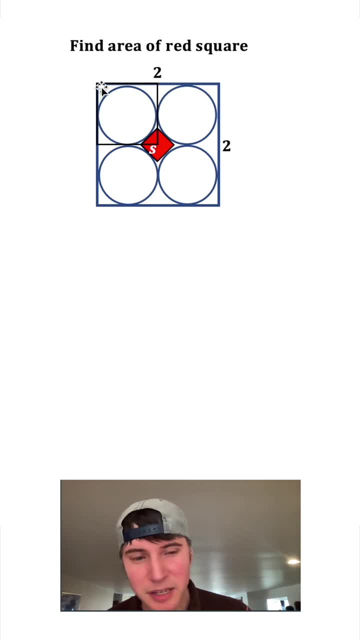 of that square, which means that I could probably flip it and get the same piece right up there just like that. So this piece should equal this piece right here. If you think about how those four squares would be cut off, both of these are exactly half of the length of S, So the two of 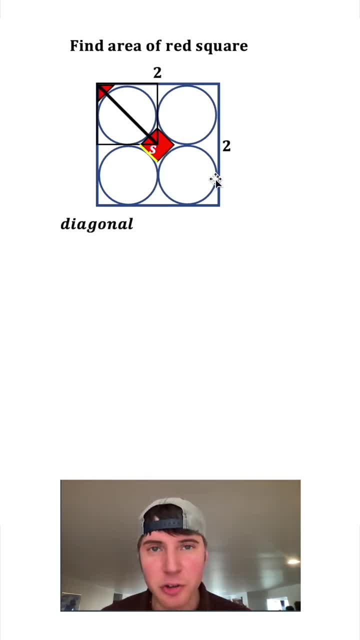 them together should just be S. Let's look at this diagonal of the square I drew in the corner. It's going to be comprised of S plus the diameter of one of these circles. How long is this diameter of this circle? Well, if we cut this side in half, each of these halves is equal to one and that half.